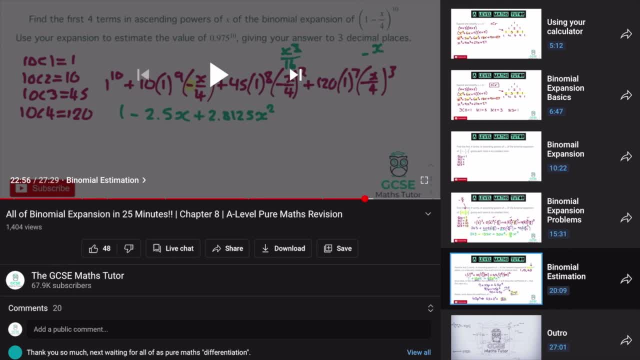 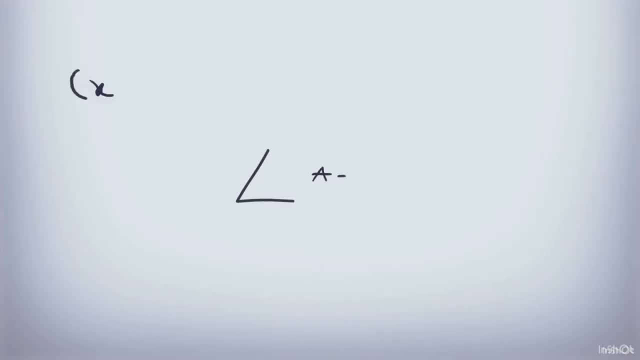 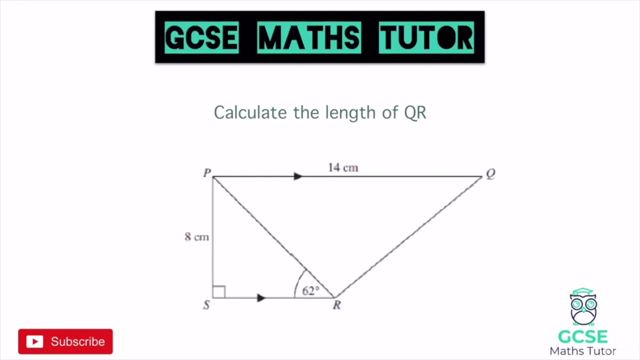 Hopefully that's useful and helpful. If you enjoy this video, please don't forget to like the video, Don't forget to share it with some of your friends. But with that being said, let's get started. Something a little bit different here. It says: calculate the length of QR. Now, QR is this length. 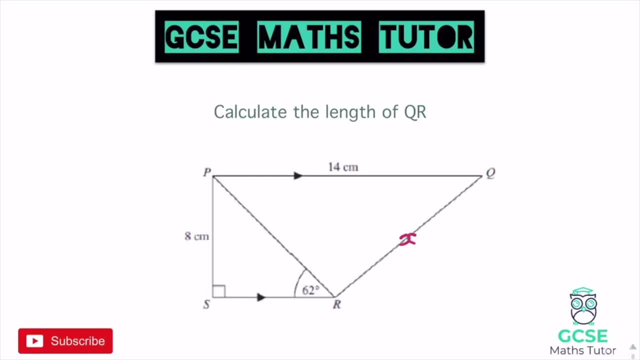 over here, So let's label that. There we go. That's QR. Now, at the moment, we don't have the opposite angle. In fact, we don't really have much in this triangle. We have the 14 and that is. 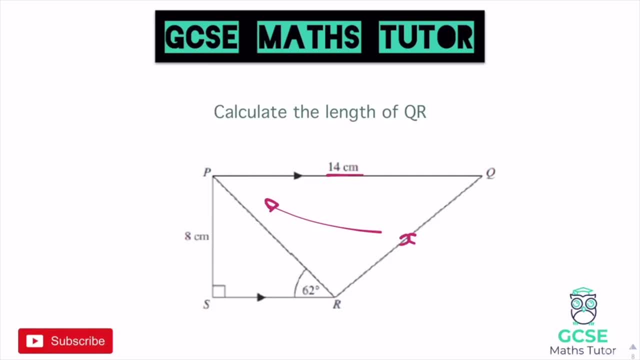 actually it, But we have got these parallel lines going through here, So we're going to have to, So hopefully we're going to be looking at some parallel line rules here, So something a little bit different. And we have got this right: angled triangle, SPR on the left, there Now on the right. 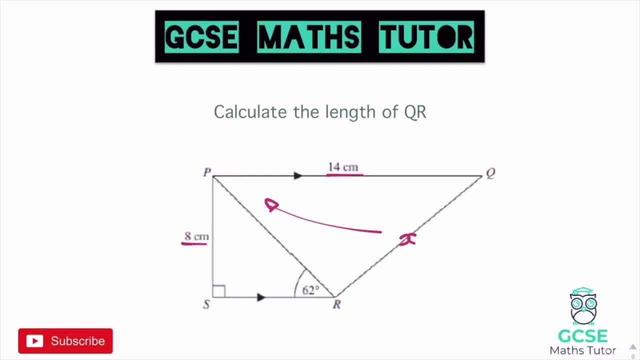 angle, triangle. we've got the length of eight and an angle, So obviously we can use Sokotoa, or potentially the sign rule or something like that, to work out one of the missing lengths. Now this one obviously stands out to me because if we can work that one out, that gives us another. 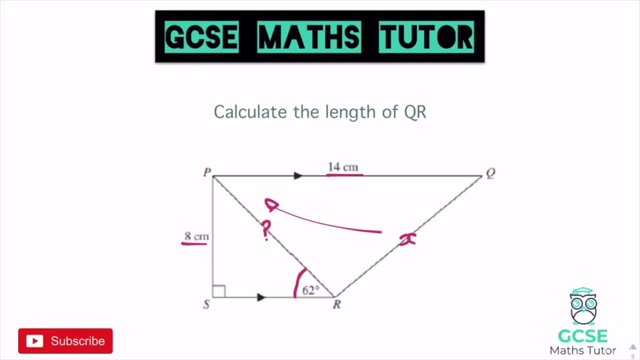 length in our little triangle on the right there. So let's think how we could do that. So, thinking about some trigonometry, again some Sokotoa. we've got this side here, which is our opposite, So we've got the opposite, and we're looking for the hypotenuse, So we can definitely use Sokotoa. 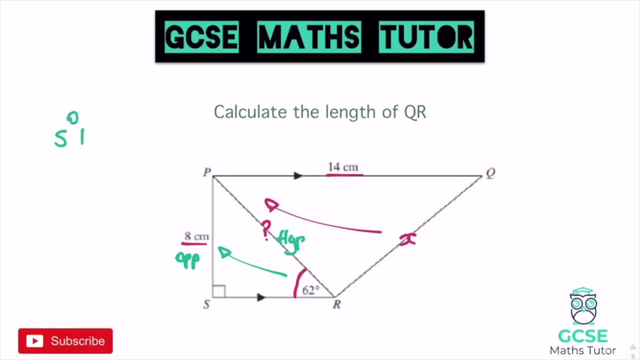 to do this Again. obviously, if you're using formula triangles, let's have a think SOH. So if we're looking for the hypotenuse, we're going to do the opposite. divided by sine: 62. So I can work that out. Definitely, Let's call that hypotenuse there. Let's just call it the. 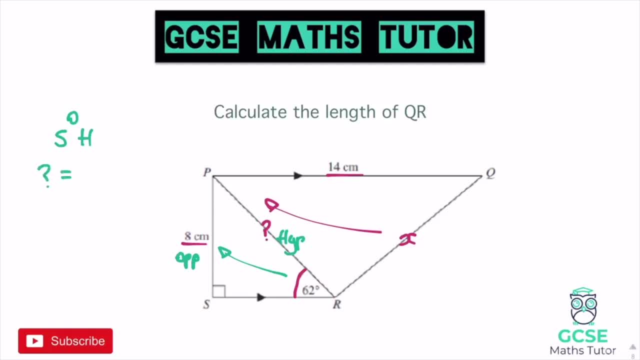 question mark, to be fair. So the question mark is going to equal the opposite, which is eight divided by sine 62. There we go, So sine 62. So let's type that in Eight divided by sine 62. And that equals 9.06.. Let's have a look So that equals. 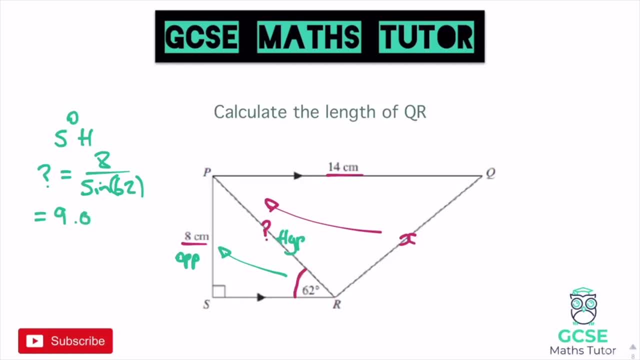 9.06.. And there's a few more decimals. I'm going to leave it like that. This question doesn't actually say let's just go for two decimal places. Let's go for that. There we go. We're going to do two decimal places, So let's label that on the diagram. So we've got 9.06.. And 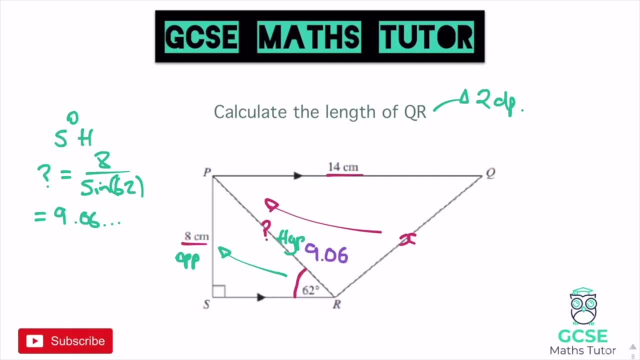 obviously, if I'm doing it to two decimal places, I should probably keep it a little bit more accurate. So it's 0.06.. So let's label that on the diagram. So we've got 9.06.. And obviously. 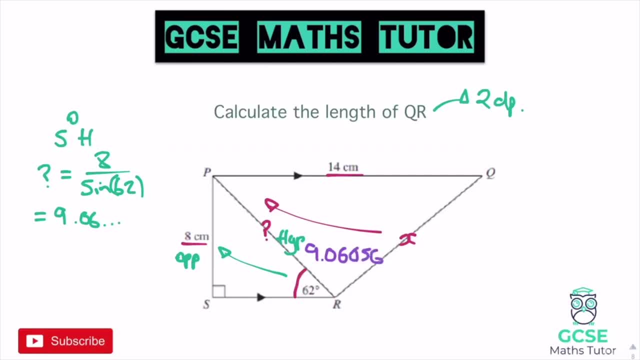 0.06.. There we go. I'm going to keep the answer on my calculator, anyway, and use that. Now let's look at this triangle on the right now. Now I have got two sides, But yeah, I'm still missing the angle opposite the one I'm looking for. So there must be something to do with the 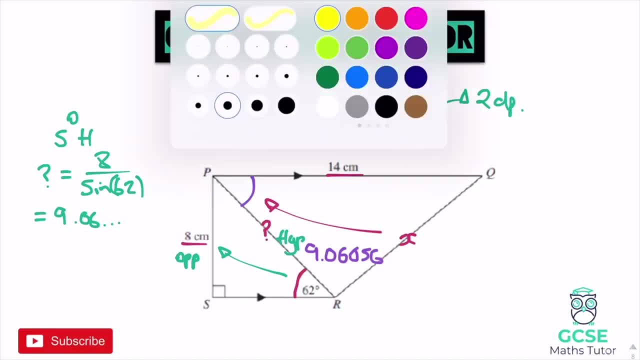 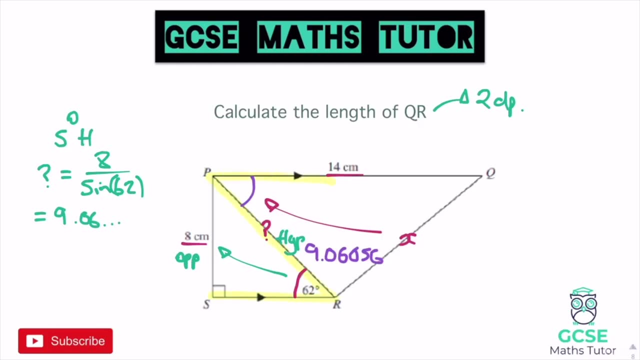 parallel lines here And if we have a look- let's just try and highlight this- We actually do have an alternate angle here. So going along a parallel line, it jumps up to here and moves along. So we've got an alternate angle there. So this particular angle here is alternate with the 62.. 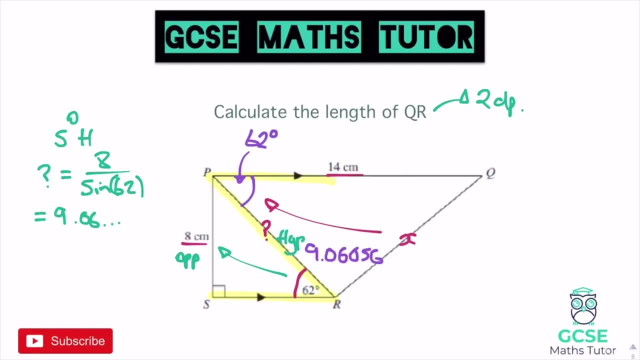 That one is also 62 degrees, And now we have all the information that we need in order to use the cosine rule. So opposite that we've got the little a, So this would be our big A, And then these will be our B and C. Let's have a look, And the one that we've just made there will be our C, So we 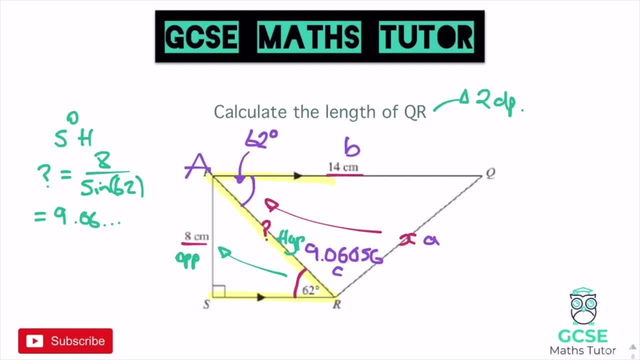 can type that straight into the cosine rule, Obviously not looking at angles here, But we might be looking at angles potentially. But this one's looking for a side length. So a squared equals b squared, So 14 squared plus c squared, which is 9.06.. And again, I'm going to leave that. 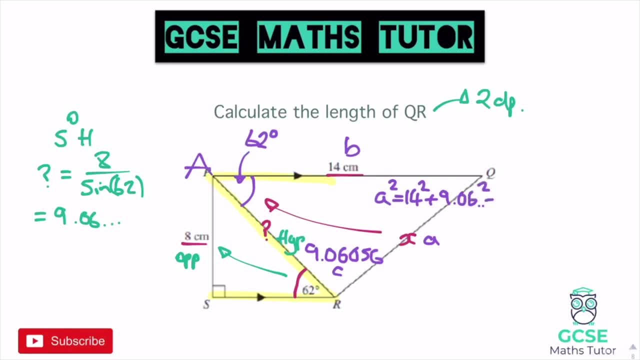 later, So I can use that in a sec. And that's squared minus 2 times 14 times c, which is this 9.06 number, Oh, 06.. There we go, And that's going to be cos 62.. Right, there we go, So let's try. 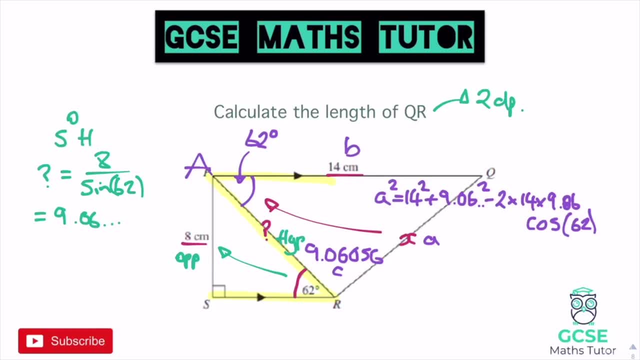 typing this in. So obviously I've left that answer in my calculator. So 14 squared plus answer, squared minus 2 times 14 times answer, And then cos 62.. Again, you can just write it down and not use the answer button if you want. I just quite. 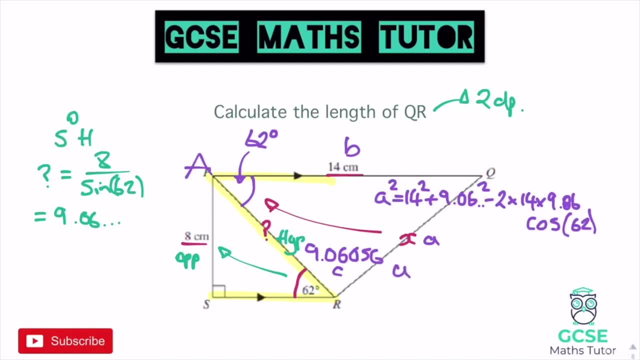 like just actually using that. So let's have a look, So let's write what we get here. So a squared equals press equals. we get 158.9908.. There we go, 9908.. And there are a few more. 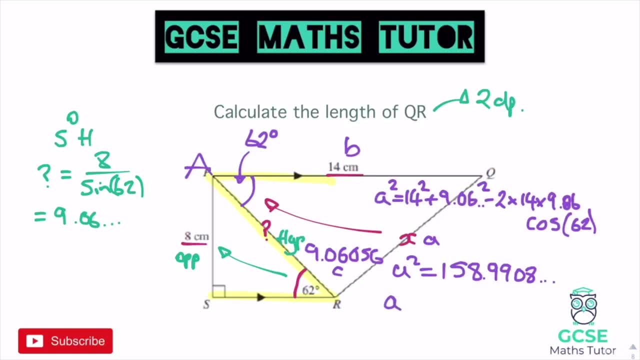 decimals, But again, we'll leave the answer on my screen. So let's square root that. So our value of a square root answer, And that leaves us with a final value here of 12.6.. 609, with a few more decimals, But if we do have that, two decimal places for this question. 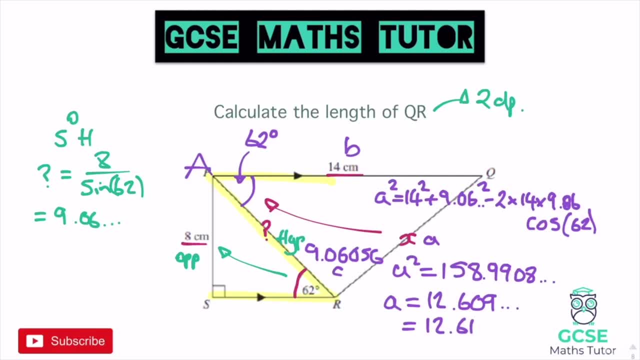 that'd be 12.61.. And this is all about centimetres. There we go, So 12.61 centimetres our final answer. So obviously a lot going on in that question. We had some Sokotoa. 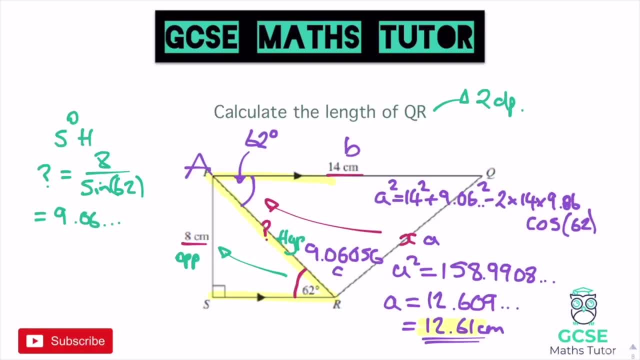 which, you know, in a different kind of question, could be looking for an angle, it could be looking for a side length, And then we had to apply some cosine rule And obviously there was a little bit of parallel lines going on in that one as well. So something a little bit. 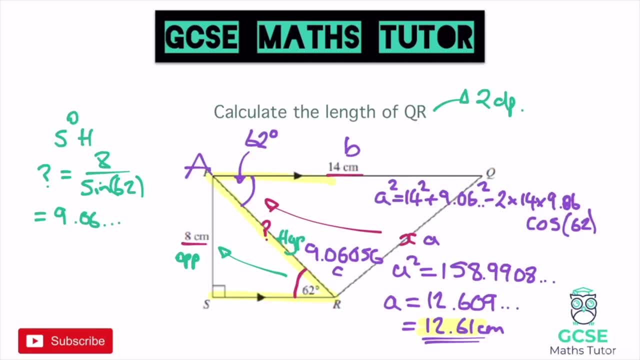 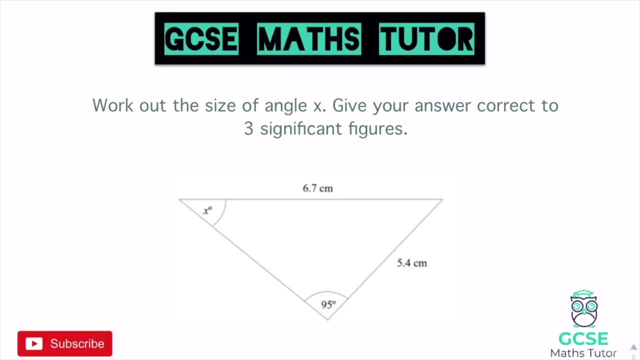 different, with a blend of different topics, But just something to be thinking about: how you could apply this topic, You know, within a different sort of setting or a different sort of diagram. that's not just a plain triangle. Okay, so this question says: work out the size of angle x. give your answer. 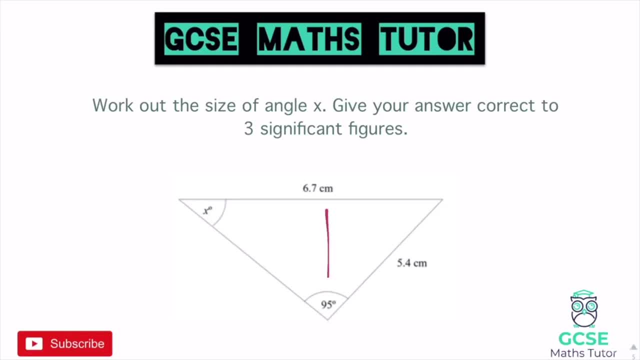 correct to three significant figures. Now again, just thinking about the question: look, I know we're finding an angle this time, But look, we have got these pair of opposites here And also we've got a pair of opposites over here. So if I just label this up just like before, 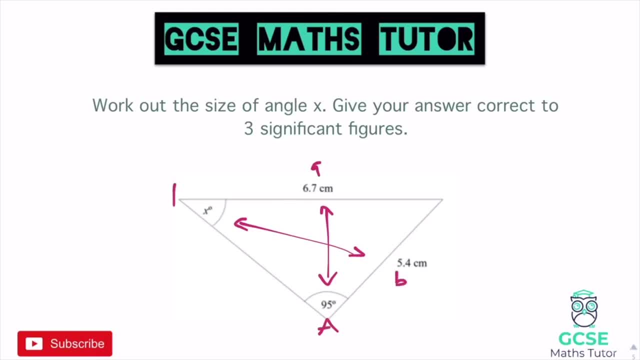 we've got A and big A and B and big B. Okay, but if I was to plug these into my sine rule, into my sine rule formula, like we did before, we'd have 6.7 over sine 95. And that would be equal to 5.4, this time over sine x. 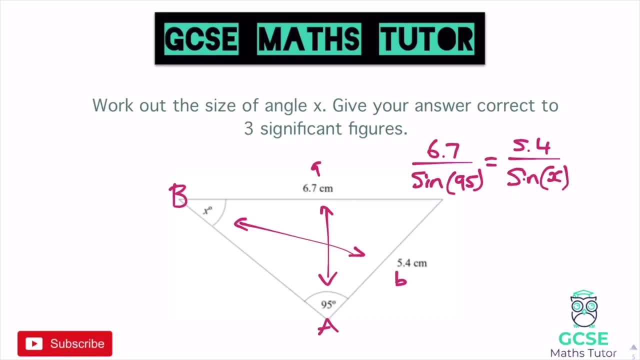 Now you can actually use the sine rule like this, And obviously we could actually do quite a bit of rearranging here to get that x on its own. But obviously what we want to do is we want to get this part on its own, this sine x part, And if we times that to, 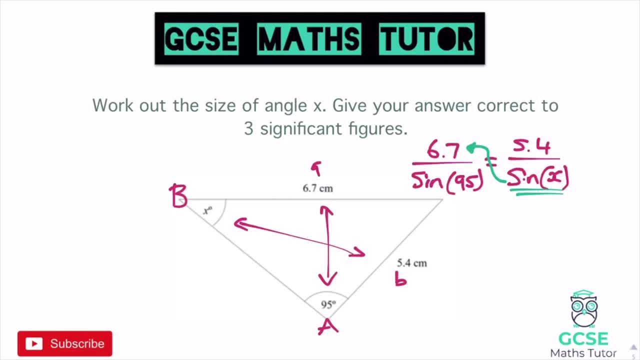 the other side. now it's going to go on to the top of the fraction here And it's not really going to be on its own in that first step. So there is a really quick step with the sine rule, obviously just to help you with the rearrangement here, And that's just to flip them over. Now the reason we 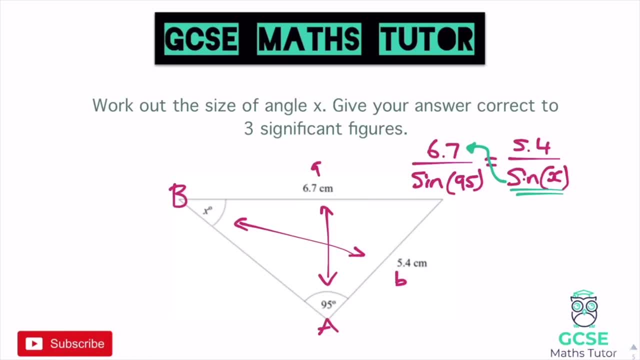 can just flip them over. if we think about a little bit of logic here, if we have two fractions that are equal to each other, let's just pick something easy like one half is equal to two quarters. Now that is a correct statement there One half is equal to two quarters. And if we flip 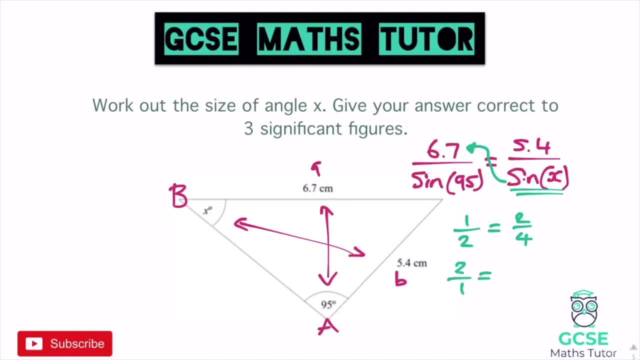 them over. we get two over one is equal to four over two. Two divided by one is two, Four divided by two is two And two equals two is again a correct statement. So you are able to flip fractions over like this. when we're equating them to each other, Obviously they equal different. 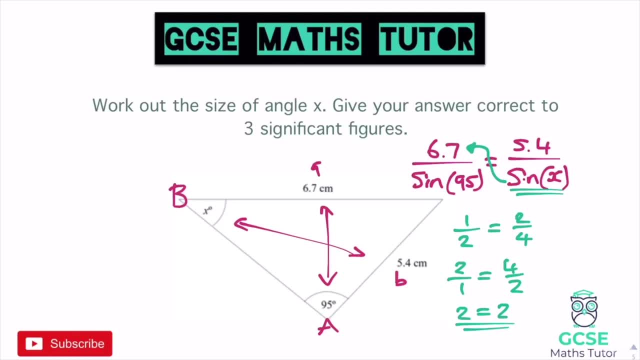 things there. but the statement is still correct. They still have to equal each other. So when we're looking for angles, all we're going to do is we're going to flip the fraction and fractions over and use the sine rule upside down, so to speak. So we've got sine a over little a is going to equal. 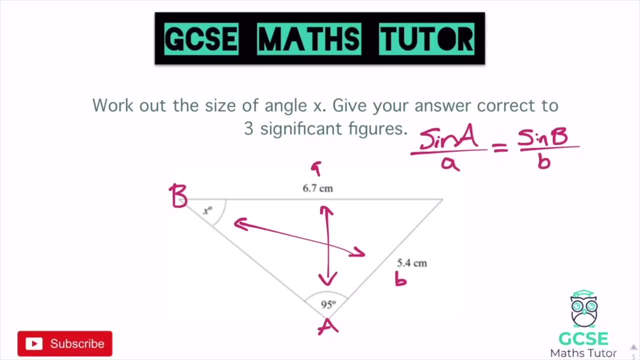 sine big B over little b. And you're going to see now, when we put the numbers in, we get to rearrange this in one step, just like we did before. So if we plug all these values in, I've got sine 95 as my big A And that's over the opposite there. 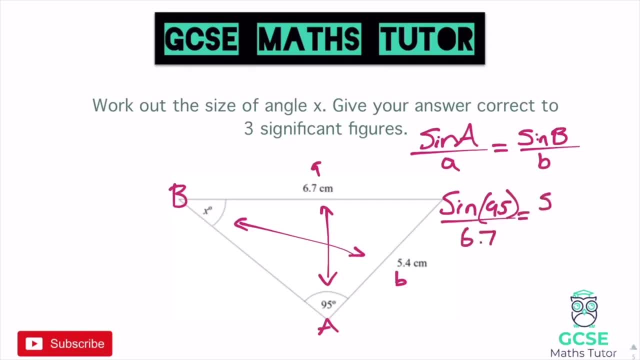 which is 6.7.. And that is equal to sine x. I'll put the x in a bracket, just like I do with the normal angles, And that is opposite the 5.4.. OK, So now we are actually able to eliminate, or. 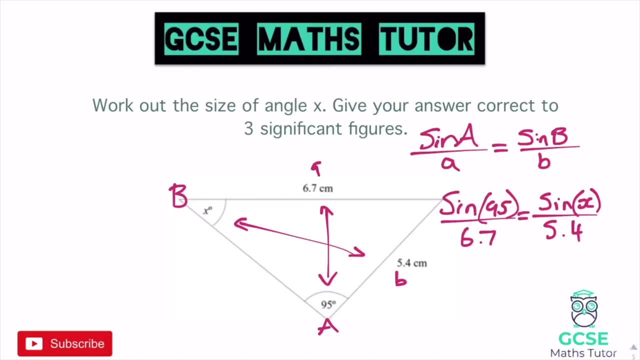 get or isolate the sine x on its own by getting rid of this 5.4 on the bottom. this divide by 5.4.. Again, just times both sides by 5.4.. So when I times this up and again, I'm going to write it. 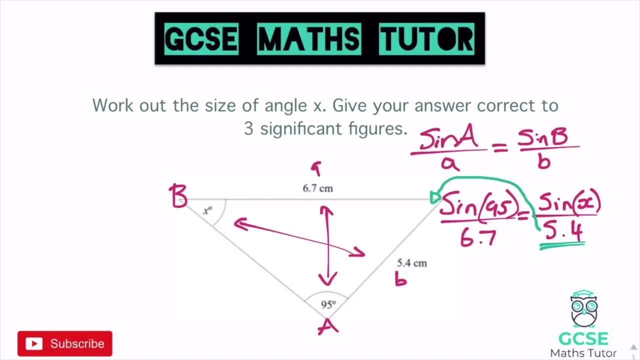 in the same way as I did before. So when I times it up to the numerator, look, I'm going to write it just at the start here And I'll write it down to start with. So that would give me 5.4 sine 95.. 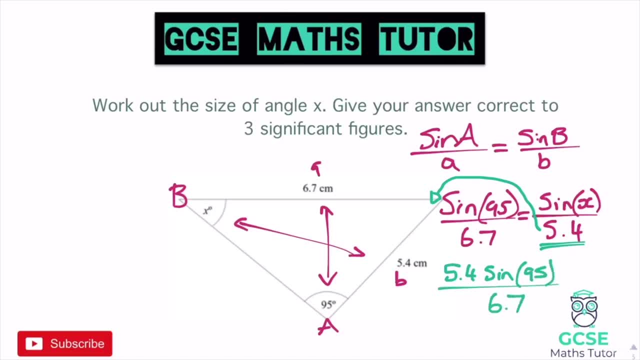 And that's over 6.7.. And that now equals sine x. There we go. So now we've got the x on its own, but it does equal sine x. Now if I type all of that into the calculator, let's see what we get. So let's type all of that in. So on the top I've got 5.4 sine 95.. 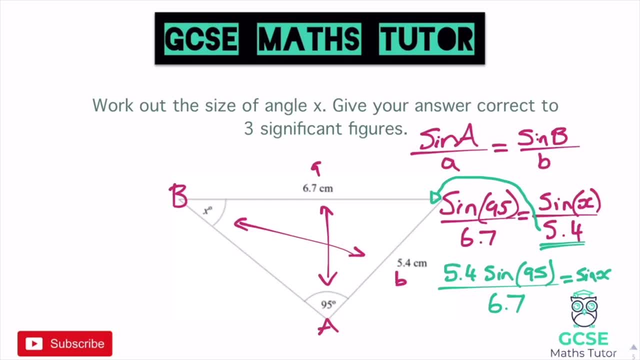 And on the bottom I've got 6.7.. And if I press equals, let's see what we get. So I get quite a long decimal, So we've got 0.802903.. And we're not going to write it all down, I'm just. 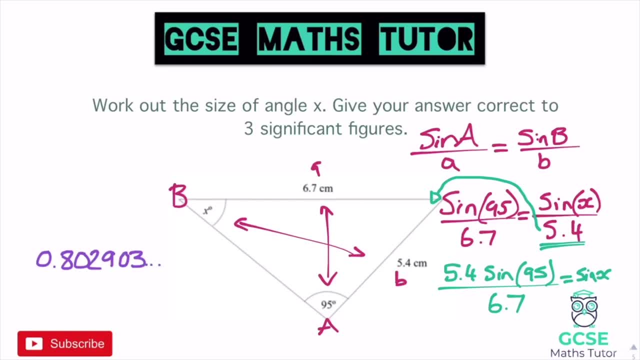 going to leave it on my calculator screen for the moment, But that is what all of this little bit equals when I type it all in Now. obviously that equals sine x. It doesn't equal x. It's not our answer. So that equals sine x, And I'll put the x back in a bracket. Now. this would hopefully. 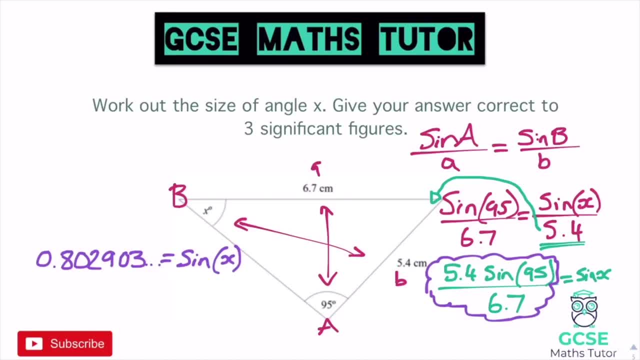 link through to normal trigonometry when we were looking at Sokotoa. If you want to separate these two parts out and obviously figure out what x is, we can do the inverse of sine. So I can press that shift sine button. It will do the inverse And that will help me just to figure out what x. 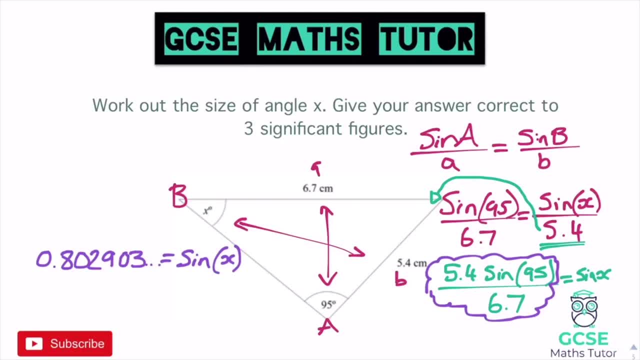 actually is and not sine x. So obviously, thinking about your normal trigonometry, press shift and then sine, And you get this sine minus 1, your inverse sine, OK, And we're going to do the inverse of this value here. that's on your calculator. 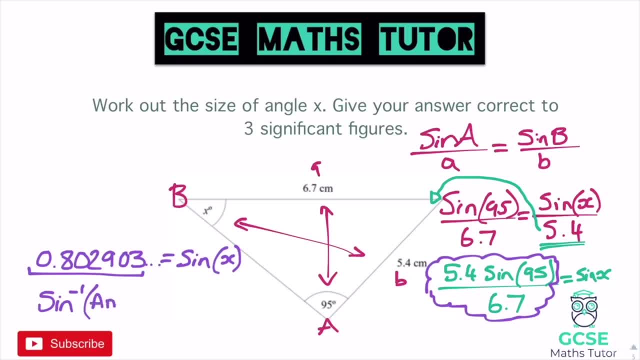 So that'll be the inverse sine. I'm just going to press the answer button, So I'm just going to write ans here rather than that decimal. But obviously that is just that decimal there that I'm writing in the bracket. You can feel free to write it all in if you want, But it seems like. 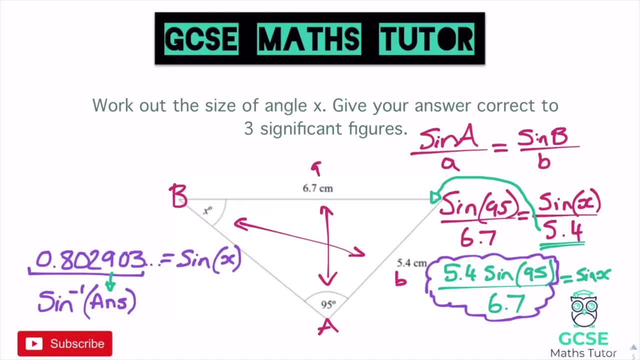 an unnecessary step when we can use our calculator a bit more efficiently here. So shift sine ans, which is next to the equals button. Click it and press equals, And it gives us the size of the angle, which is 53.408.. And a few more. 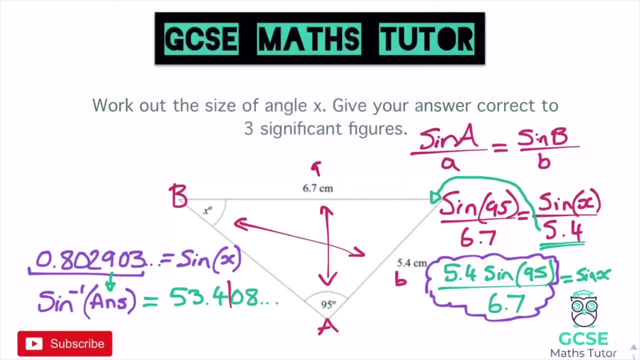 decimals, But again it wants me to round it to three significant figures, So I can chop it after the four And we get 53.5.. There we go, And this is about degrees this time. So degrees, And there's. 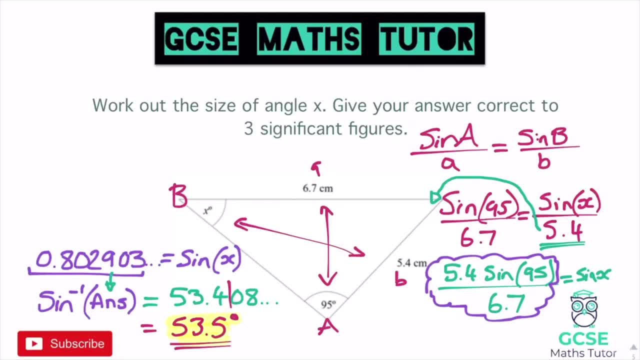 our final answer. It's obviously a very similar process in terms of the way we use the formula, But we have that final step there of using the inverse of sine to find out the size of the angle, Just like with normal trigonometry when we're looking at right-angled triangles. 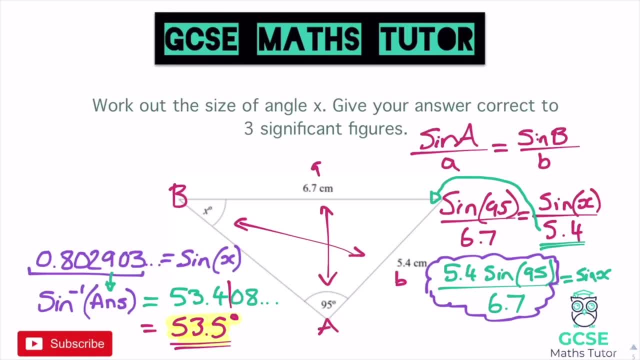 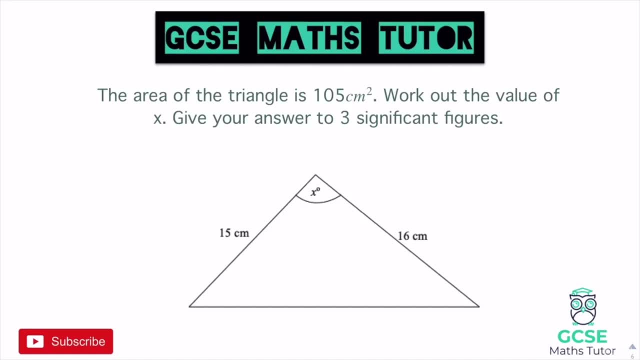 we still use that inverse of sine when we're looking for an angle. OK, so this question says the area of the triangle is 105.. Work out the value of x And in this case the value of x is the angle there sitting at the top. So if we plug these all into the formula, 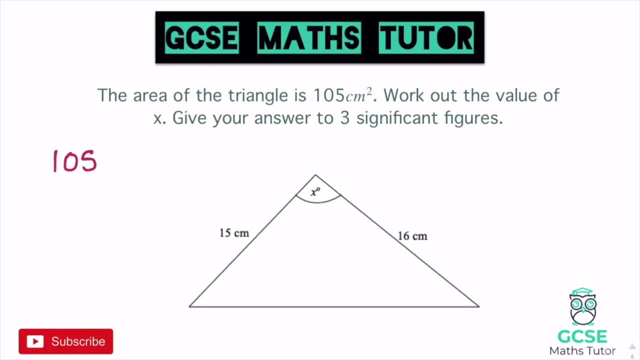 again we've got area equals, So 105 equals. There you go Half ab sine c, So let's just call that c. And then we've got r, a and b here, So it's a half times 15 times the 16 there. 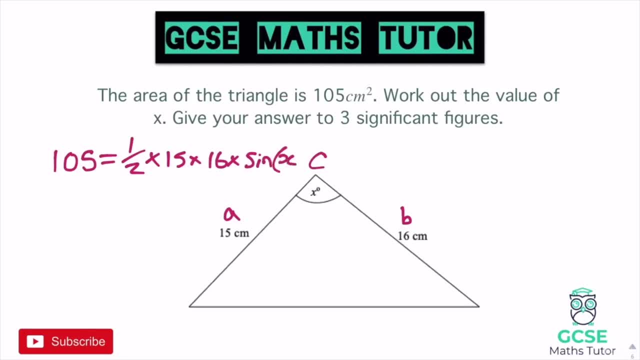 Times the sine c, And in this case that is x there, So sine x. Now again, this is quite nice. I'm going to take the quicker approach. I'm going to divide all these pieces straight over. A half times 15 times 16.. Again, you could work that out and divide it over, But I'm just going to write. 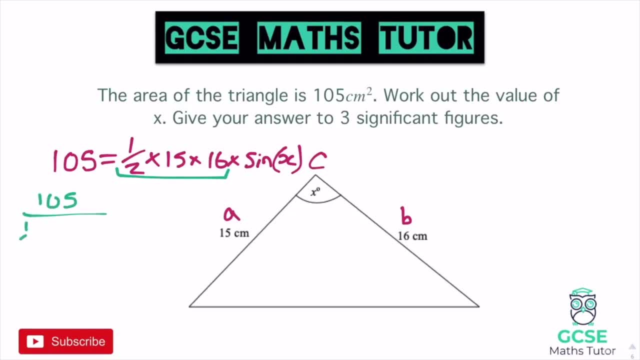 all the work in out. So I'm going to do 105.. I'm going to divide it by a half times 15 times 16. And that's going to equal sine c or sine x in this case. There we go. So let's type that in. So 105 on the top. 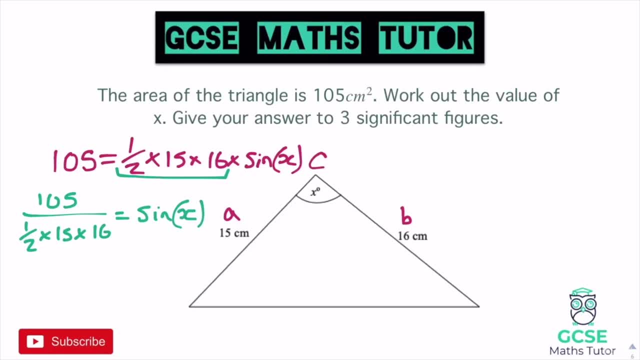 And we've got 0.5 times 15, times 16 on the bottom And it gives us 7 eighths, or the decimal 0.875.. So 0.875 equals sine x, And again we want to know the value of x here. So, just like with all, 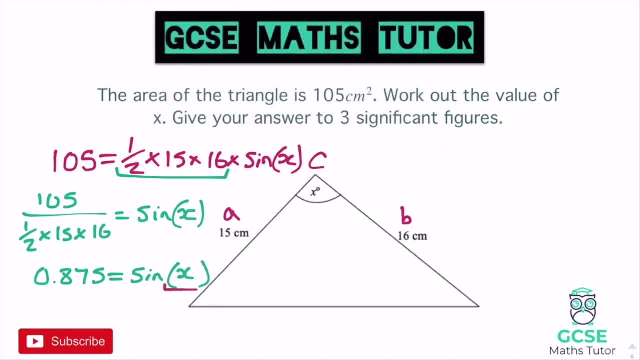 the other trigonometry that we've looked at. when you're trying to find the actual x piece here or isolate and find the angle, we want to do the inverse of sine. So I'm going to leave that 0.875 on the calculator Again, it's not too difficult to type that in, But I'm just going to leave it in. 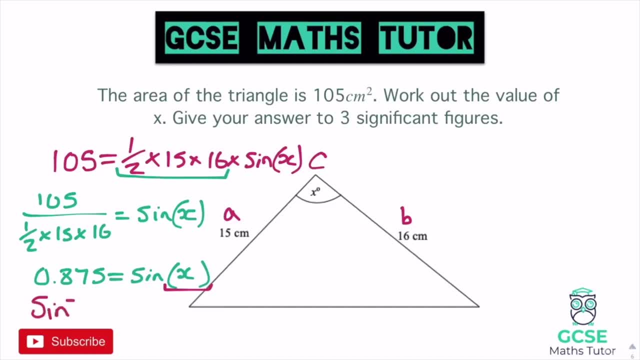 because it could be a nasty one. I'm going to do shift sine, which brings up my sine minus 1, my inverse of sine, And I'm going to put my answer in. So I'm just going to press the answer button. 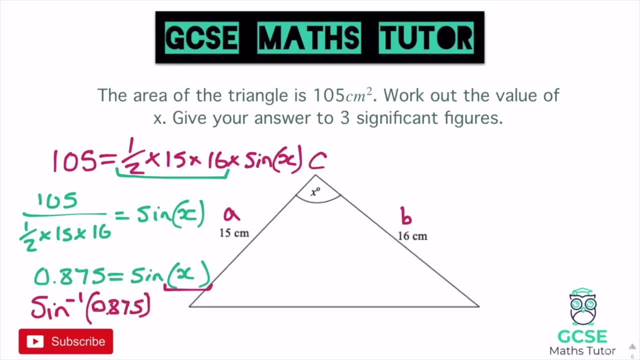 But I'm just going to put 0.875 in there. There we go. So I want to know what angle gives me that value there for sine. So if I type that in, so shift sine And I'll press the answer button and 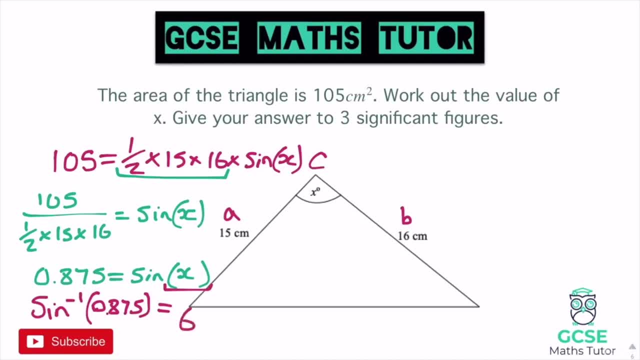 close my bracket And here we go. I'll get my degrees here, which is 61.0449.. There's a few more decimals, But again, we are rounding this now to three significant figures, as it says up there. So that's the 0.. 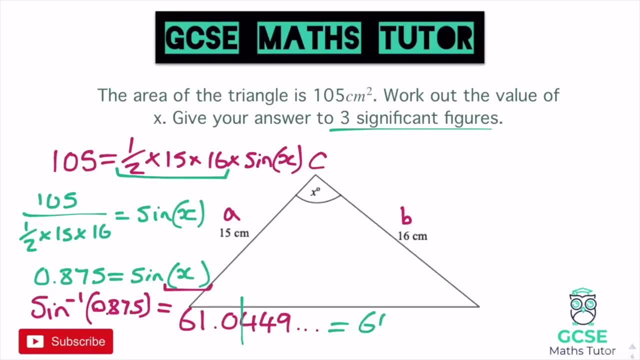 And again that 4 is not big enough to round it up. So that's going to be 61 point And I'm going to keep the 0 in there, as it wants three significant figures. It's just indicating that it wasn't big enough to round it up there. So 61.0 degrees for that question. 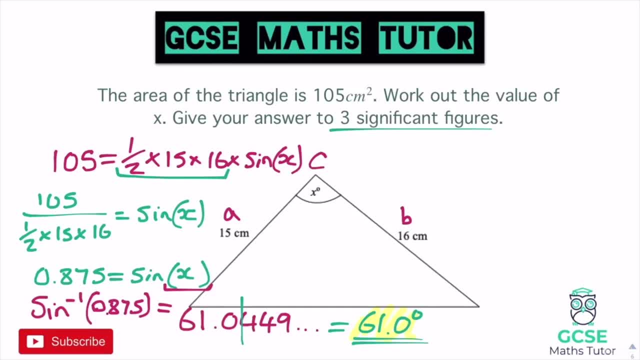 Very similar process, look. But when you're finding an angle, just like all forms of trigonometry, we have to do that inverse at the end. So the shift sine to get the inverse to get the angle. OK. so there we go. There's two examples. Just plugging it into the formula, dividing everything. 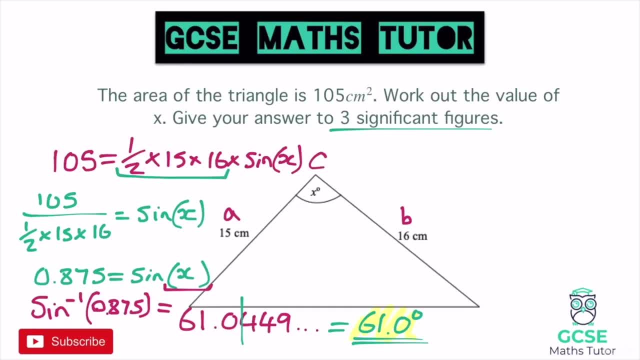 over to the other side step by step, Or you can do it all in one jump, like I've done on this one. And then obviously just remember, when you're looking for an angle you have to do that shift sine to get the inverse there to get the angle. 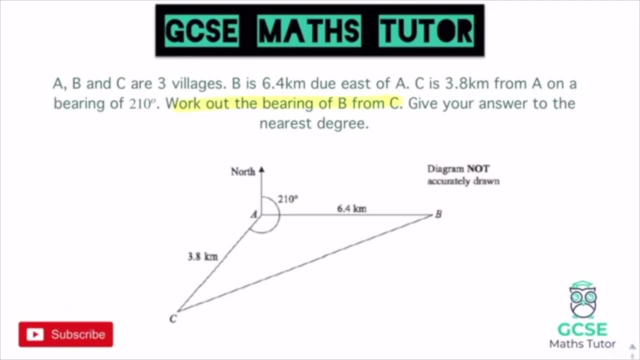 But work out the bearing from B to C. So if we have a look at the bearing from B to C- sorry, B from C- then we're going to be having a look at this angle down here, how to get to B from point C. So we're going to try and see if we can work out this angle here. 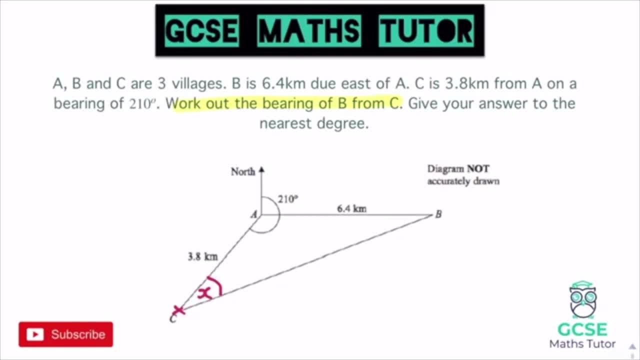 Now we're going to apply a lot of the methods that we did previously in order to get this because, thinking about finding an angle within a non-right angled triangle, we can obviously apply the sine rule or the cosine rule Now looking at this, if we have a look at this as a triangle. so obviously just highlight some of 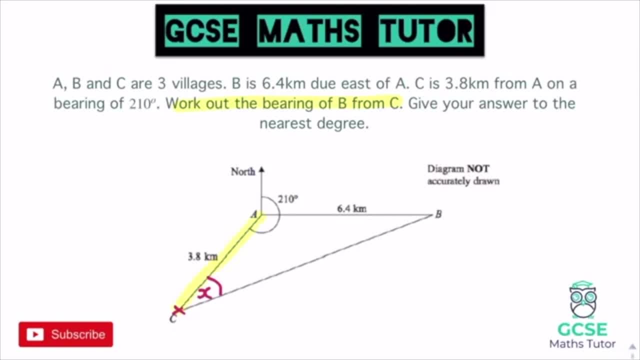 this. we've obviously got this length here, This length here. we know we can work out this angle here. OK, this one here. let me just put I was going to put a little question mark in there. There we go. We know we can work this one out And then thinking about how we might apply some. 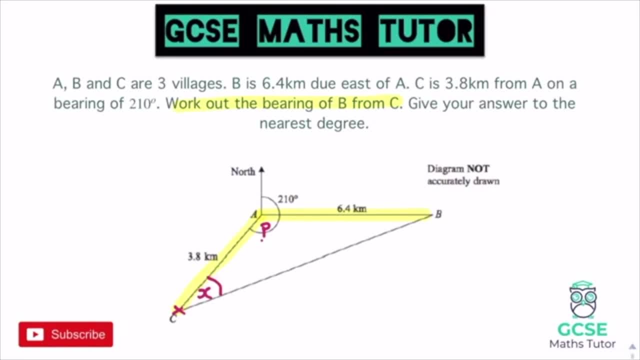 cosine rule or some sine rule to that or something. how could we actually go about that? Now, we worked out that angle, We worked out this length And as long as I have those two, I can actually do a bit of sine rule. OK, we can do the opposite pairs here and we'll have an. 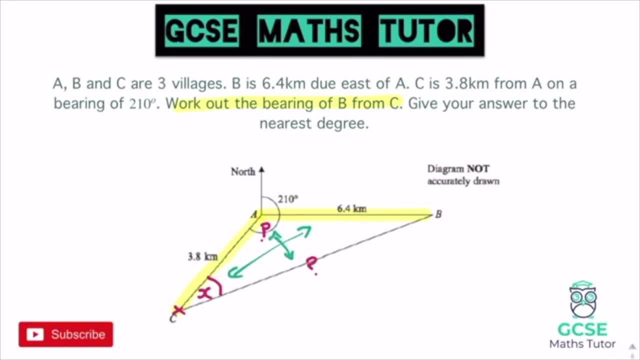 opposite pair there, Or we could actually use the other opposite pair if we were to find the other angle, potentially, But the quickest way is going to be for us to just look at a pair that we already have straight away. So, actually, if we go about doing some of those steps that we did previously, 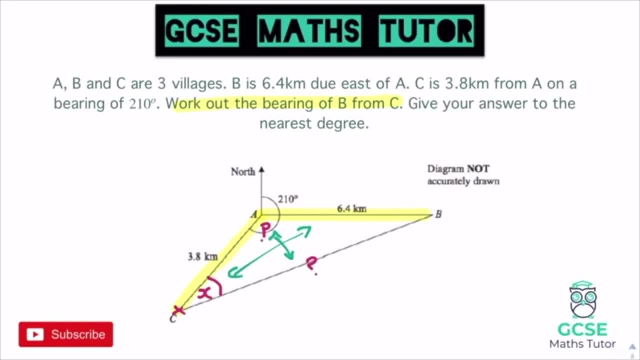 we should be able to work out any distance or any angle within this triangle. Let's have a look at actually going about doing that And some of the steps we're going to do pretty quick here because we have already looked at this particular question in this particular 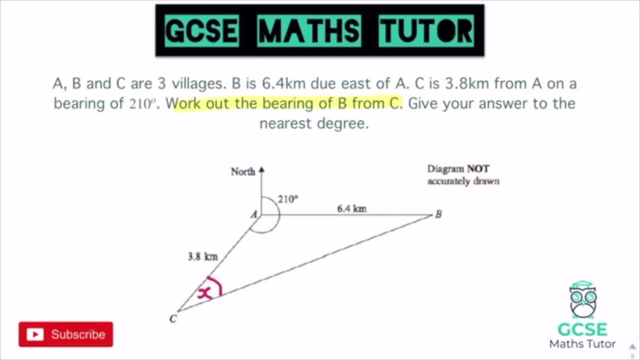 example. But let's have a look at how we would go about it. So obviously it said it's due east. So we obviously knew this was 90. And we'd already done 210.. Take away the 90 to get that little. 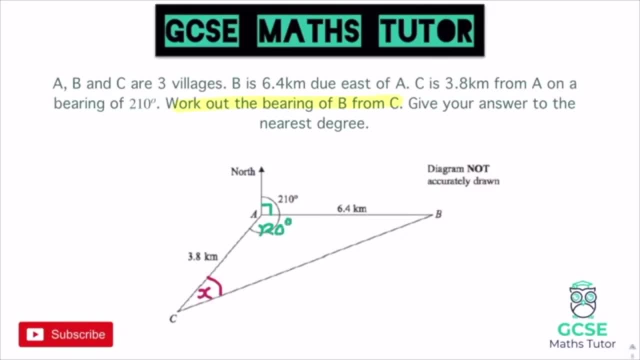 angle inside the triangle, which was 120 degrees. And there we are, So we already know that was 120.. We then use the cosine rule to get this one here. So we did a squared equals. let's have a look. the other two lengths squared So we had 6.4 squared plus 3.8 squared. 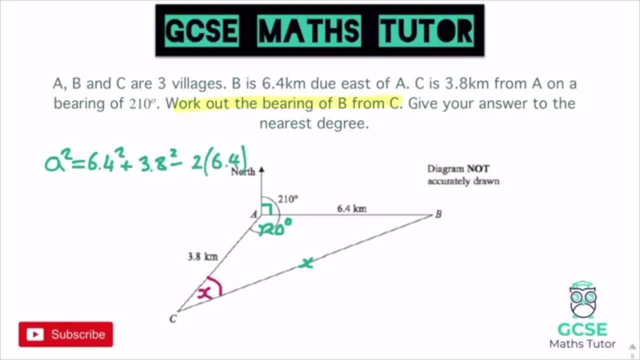 times 6.4, times 3.8.. There we are cos 120.. Right, there we go. So I'm going to square root that all in one go just to get the value of a nice and quick. So I'm going to do a square root. 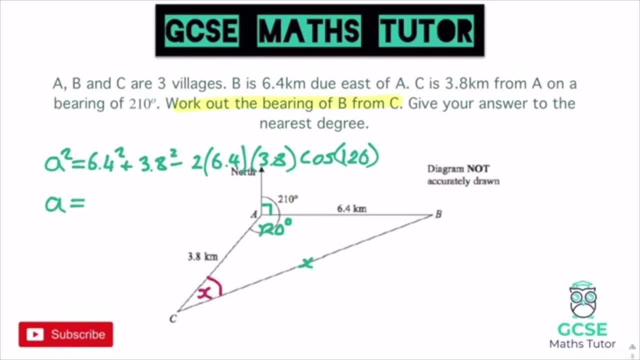 of 6.4 squared plus 3.8 squared minus 2 times 6.4 times 3.8, cos 120.. Pressing equals, there we go. We get our value here, which was 8.9286.. 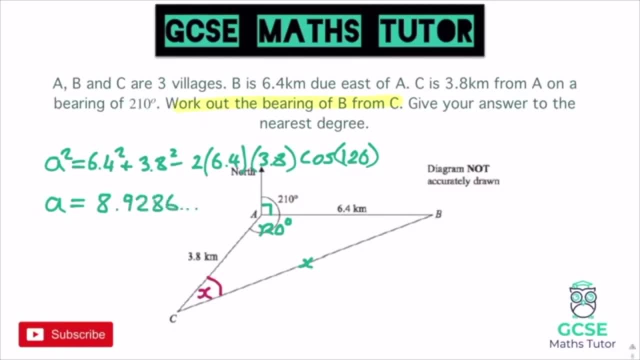 There we go: 9286.. There's a few more decimals after that, but I'm just going to leave it as it is Anyone's answer to the nearest degree here. But if I label that on there, then so let's get rid of the x And we've got 8.9286.. A few more decimals, There we go. 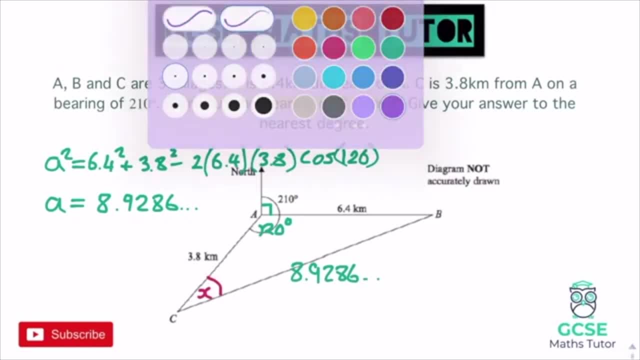 it's our little value there. So now, now that we've got that, now we've used the cosine rule, we've got a pair of opposites Here. we are those two, And we've got another pair of opposites over. 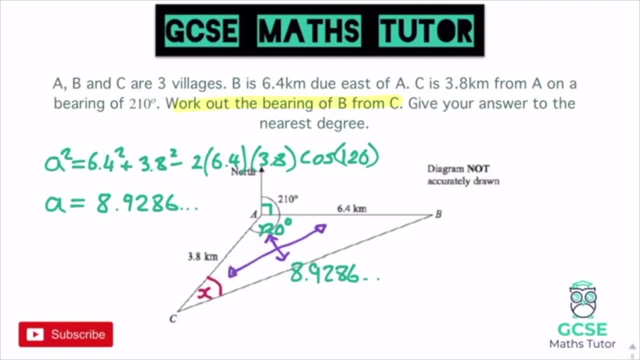 here opposite the angle that we're looking for. So we can use the sine rule now to work out what are the angles. And let's just imagine we could also do the same thing if we wanted to work out this angle over here. Obviously, once we've got one of the angles, we can work out all of the 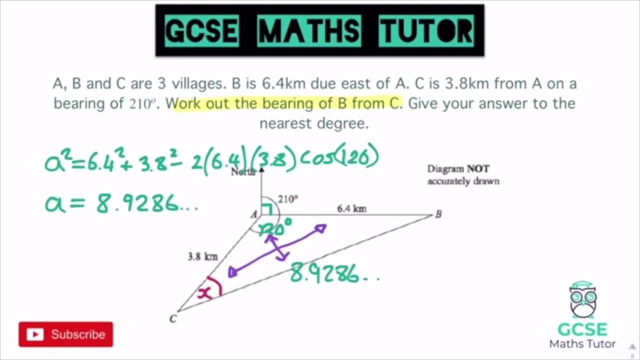 angles anyway, because it's angles in a triangle. But there we go. let's get rid of that. We'll focus on the actual angle that we're looking for. So when we're looking for an angle, we're going to use the upside down version of the sine rule. So we've got sine A over A equals sine B over B. 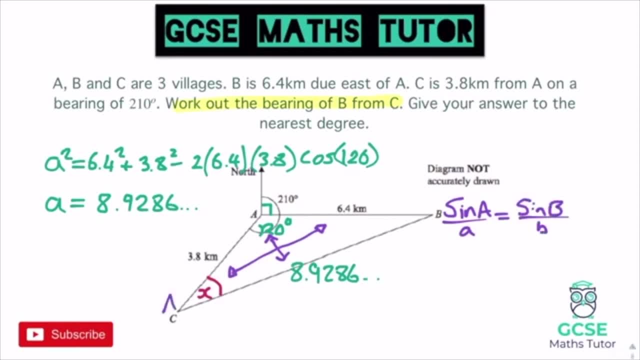 There we go sine B over B. So let's just apply all these. So let's say this is A and this is little A, And we'll say: this is B and this is my little B. Obviously, you can swap and change them. 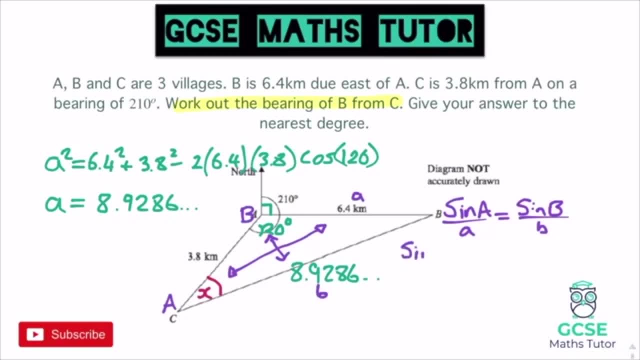 if you want. So we've got sine X, our sine A, So sine X over 6.4.. What's opposite that? There we go, And that is equal to sine 120.. And that is over. what's opposite the 120, the new 8.9286 that we've. 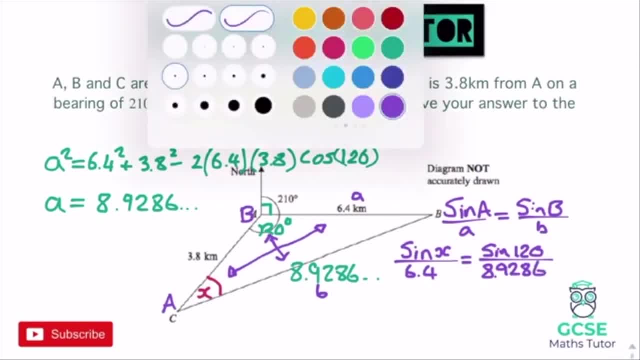 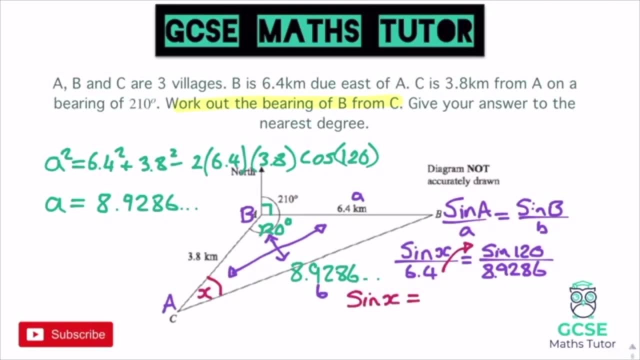 just worked out Right so we can rearrange that. We want to times that 6.4.. Up to the other side, up to the top there, So we'll have: sine X is equal to 6.4 sine 120. 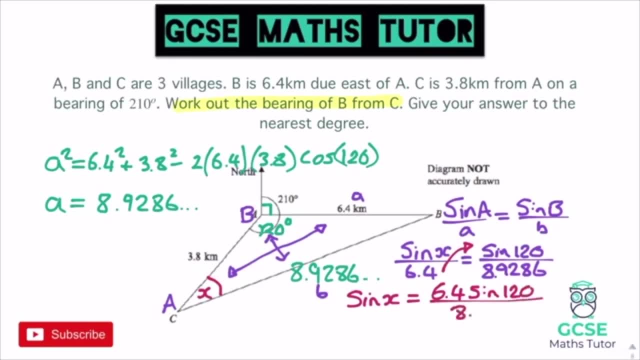 all over the 8.9286.. There we go, So let's work that out using the fraction button. So 6.4 sine 120.. And that's all over 8.9286.. I probably could have used the answer button there just to make. 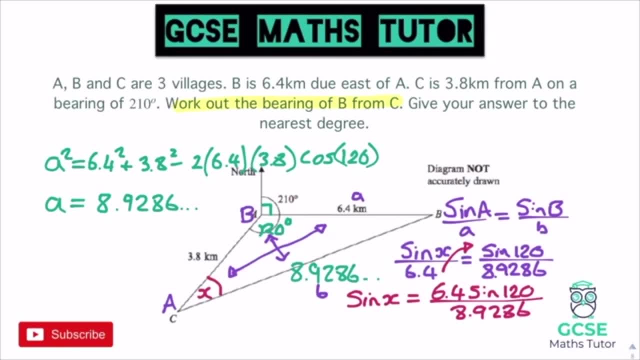 sure this is super accurate. I've left it to four decimal places. It's not going to make much of an impact on my answer here. So we've got our value of sine X. So we get sine X equals 0.6207.. And again, a few more decimals. 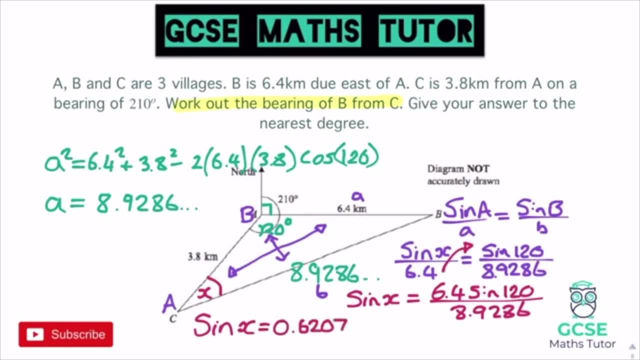 6207.. But we want to find the value of X, So I'm going to do the inverse of sine, So I'm going to get X equals. remember we're doing sine minus 1 here. so shift sine, answer And we get 38.37. 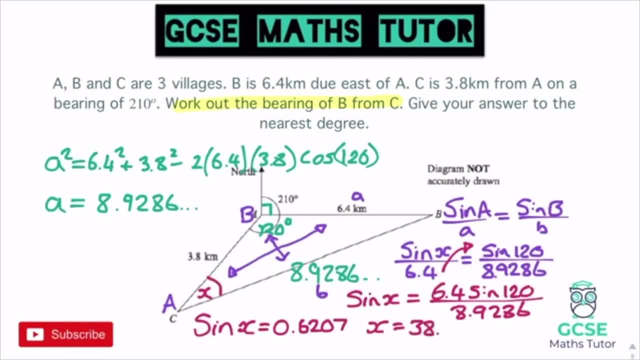 degrees 38.37.. A few more decimals after that, But it wants it to the nearest degree. So to the nearest degree. X is going to equal 38 degrees. There we go. So 38 degrees, There we are. And it does say: 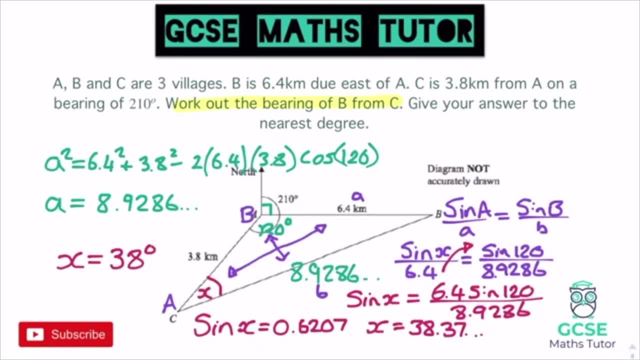 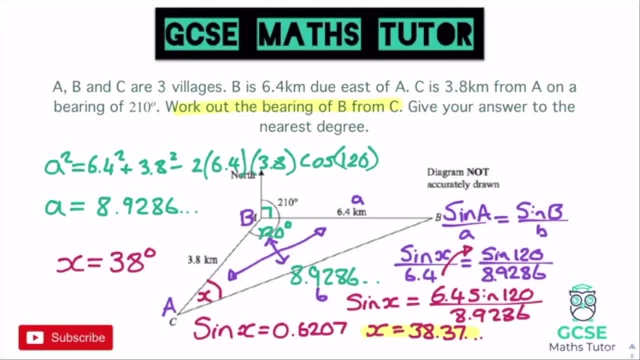 work it out as a bearing. So there's one more little step on here. Let's just highlight that. down there There's our last little bit of working out Right. So now we've got that, the angle there is 38 degrees. We need to think about this in terms of a bearing. Now remember the question. 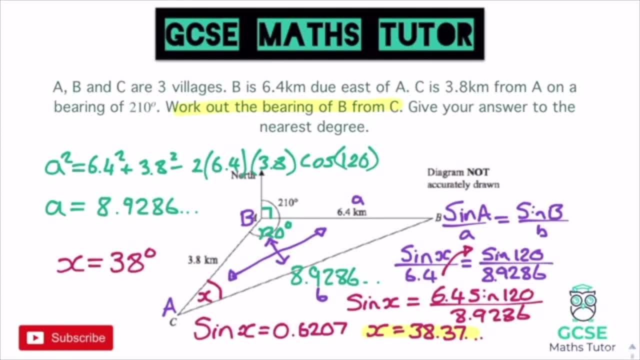 said the bearing of B from C. If we look back at C, there's quite a lot of drawing here, So I might get rid of some of this stuff in a second. And we draw our north line in. This is where this question gets really quite. 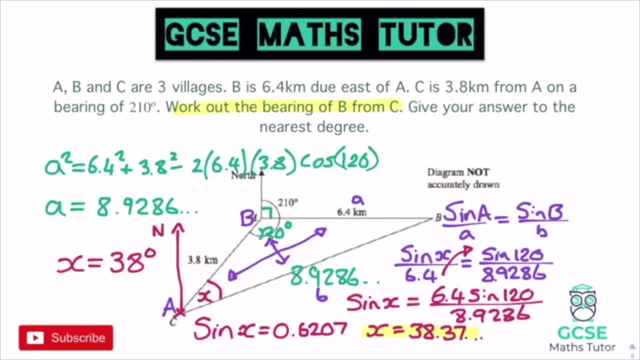 tricky Because obviously we've got the 38 degrees. We kind of feel like that question's finished there. But it wants the bearing of B from C. So really what we have to have a look at is the total angle from north, Because it is a bearing, not just an angle. So we need to know, not just the. 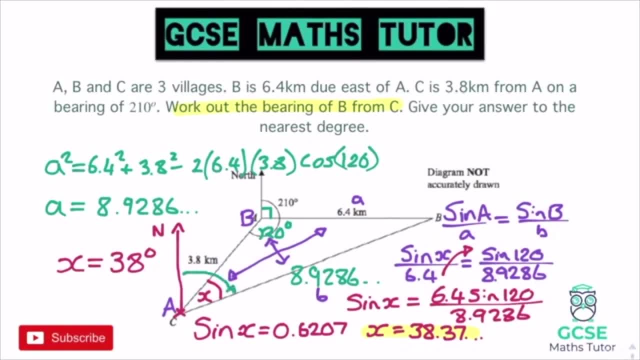 value of X there, which is now 38, but the full angle here. So if we get rid of that X, we'll put our 38 in there. as we've worked that out, There we go, And we also need to work out what the rest of the missing angle is there. 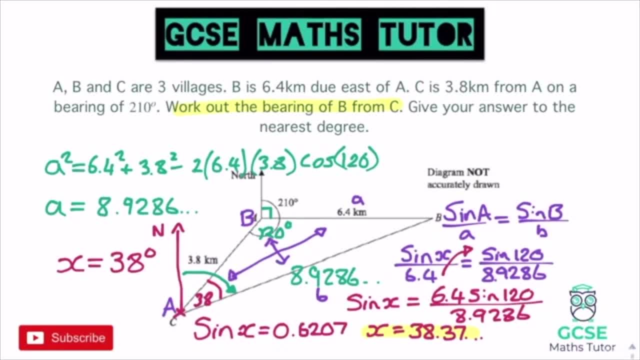 Now there's nothing actually too tricky with working that out, But I'm just going to get rid of some of this working so we can kind of see this a little better And we'll have a think about how we're going to actually approach this. Just a final step here, So. 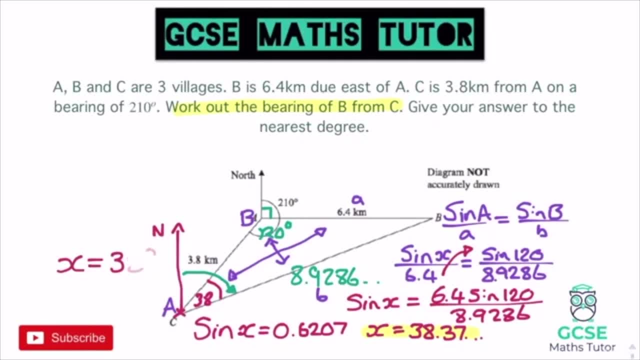 we get rid of that. We've got all of this information now. We know that X is 38. We've worked that out And let's just get rid of some of this writing here. Get rid of some of that. There we go, Right. So hopefully you can see this a little bit more clearly now. 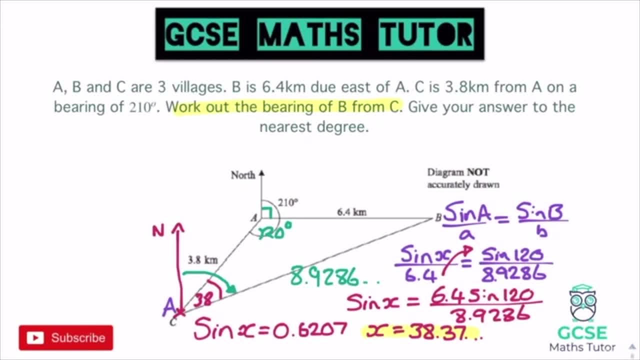 So, in order to find that angle, look, if we think about one of the earlier steps we looked at in one of the bearings videos and that is just thinking about the angles here within these two north lines, within these parallel lines, Obviously those angles there are co-interior, So we can find this angle here, if we can find. 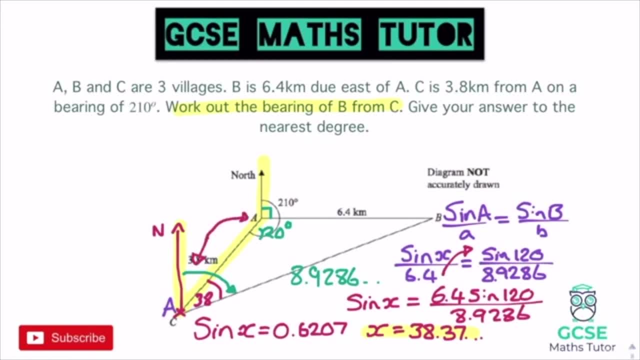 this angle here, because those two add up to 180.. Now that angle there on the right is not too difficult to find because we've got two of the other angles. We've got that this one's 90 and we've got that this one's 120.. We're already told that the full angle 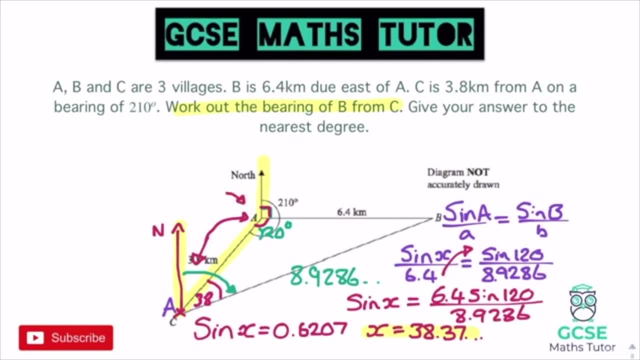 there was 210.. So we can find this one here by taking that away from 360.. So 360, take away the 210 that's given to us and that leaves us with 150 degrees for that angle there. So let's just get rid of some of this working again. So if that angle there is 150, there. 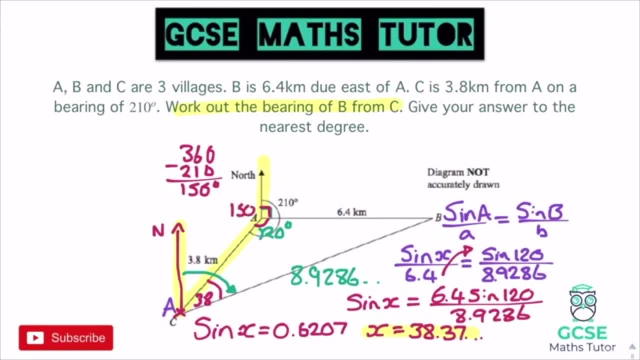 we are. that's 150 degrees. Given that these two here now add up to 180, that means that this little angle here has to be 30. There we go: 150 plus the 30 makes them add up to 180, as they are co-interior Right. so now we've got that, that is 30. We can now get. 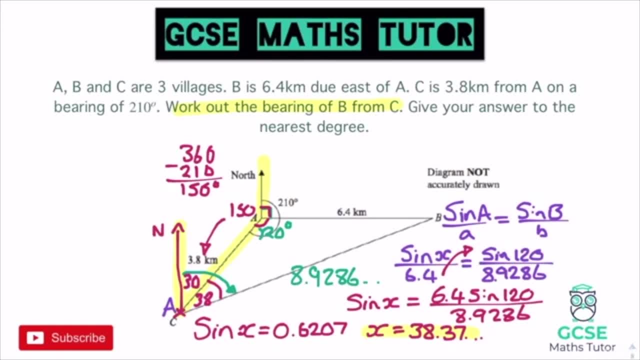 the total angle of those two. So let's just get rid of some of this again And let's just think about what we've got there. There we go, So with our full bearing, then from north going clockwise from to B- sorry, bearing of B- from C. So from C here down to that line. 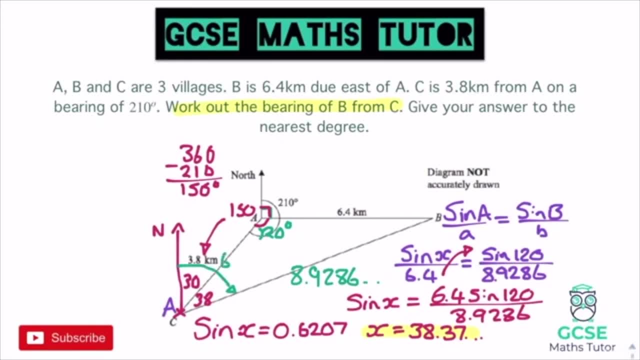 with the B on that total angle, there is going to be 68 degrees. Right there we go. So the full angle there is going to be 68 degrees. Right there we go. So the full angle there, the full bearing, is 68 degrees. So obviously our answer is going to be 68 degrees. but 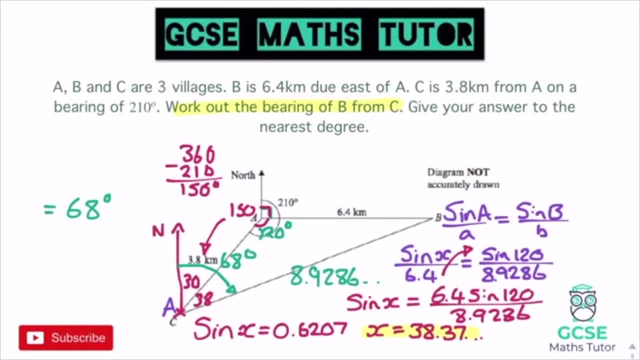 not forgetting, as well as a final step, it's got to have three digits, So that's going to be 0, 68 degrees, And not forgetting that in the final step there It's always horrible when you finish up a question like this: you've done all this, working out all those steps. 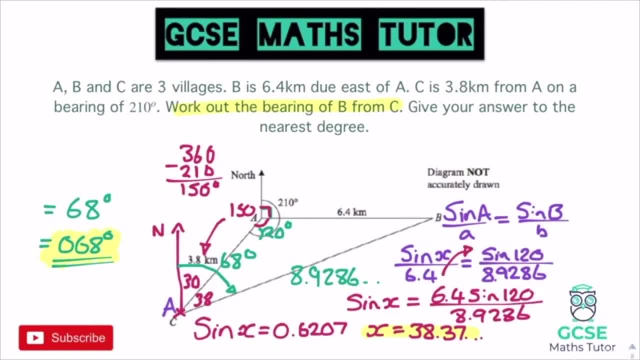 and then you just miss out that one last little mark, making sure it's got three digits. But that is our final answer: 068.. So there's a lot going on in that question. We had a lot of bearings rules then we had. 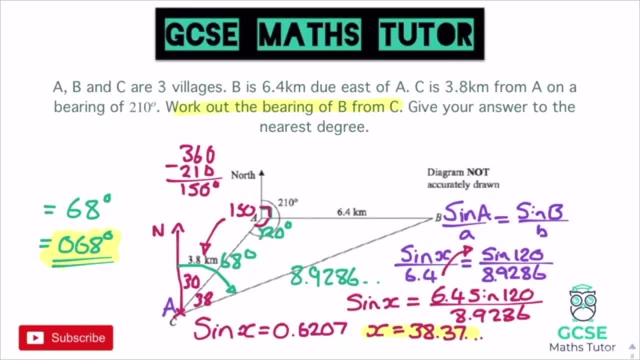 cosine rules, sine rules, And then obviously finding the missing angles using a few more bearings and actually combining that and all and actually making sure you get the final answer in the end with three digits. There's a hell of a lot to think about in that question there, And there's a lot 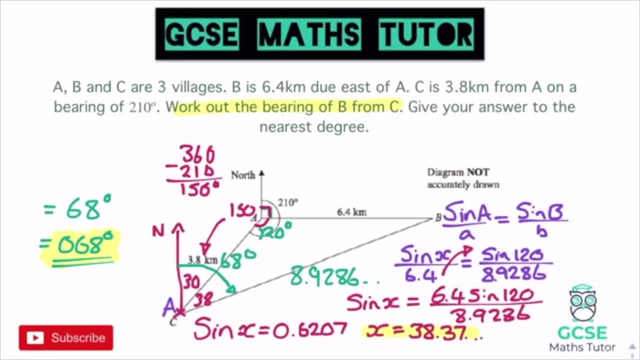 going on and a lot of maths that you've got to be thinking outside the box with as well, because obviously you've got to be able to sit and think in the moment: what do I need to use here? Do I need to use the cosine rule? Do I need to use the sine rule? So always. 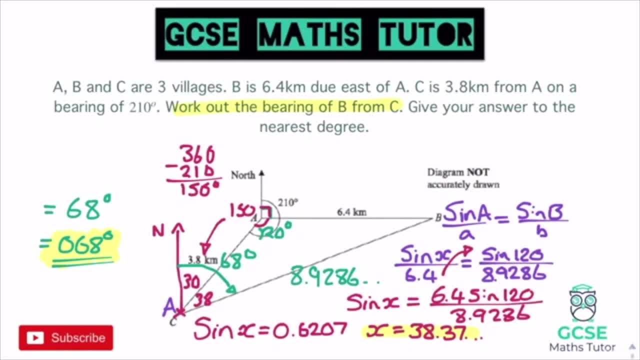 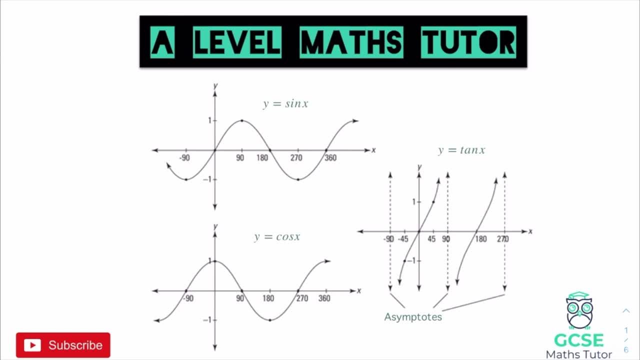 just try and break it down in steps and have a think about what you're actually trying to find and where you're going with the question. Okay, so when it comes to trigonometric identities equations, it is essential that you know the trigonometric graphs. So, as you can see, 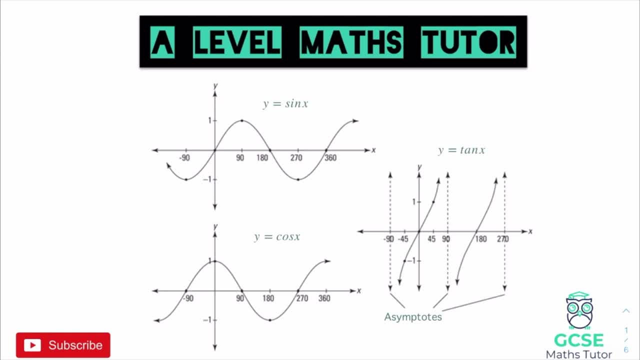 on the screen. I have three of the trigonometric graphs and it's very important that you are able to do a sketch of these. These are quite accurate- the ones that I've done on the screen- but you need to be able to draw a sketch of them. So you need to know that for y equals. 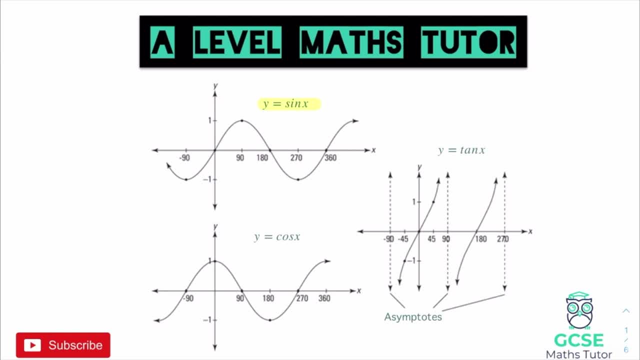 sine x, it goes in the origin, and then we have these waves that go up and over every 90, or up and under every 90. So it goes over the 90,, down through the 180.. Under the 270, and then back through the 360. And this graph here goes on infinitely. 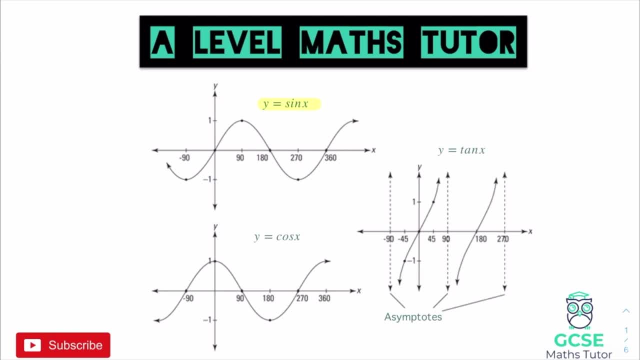 to the left and right of the y-axis. but we need to know how to draw a sketch of that and you're going to see why in some later questions. For the one below for the cos graph, this has just been translated, or it's the sine. 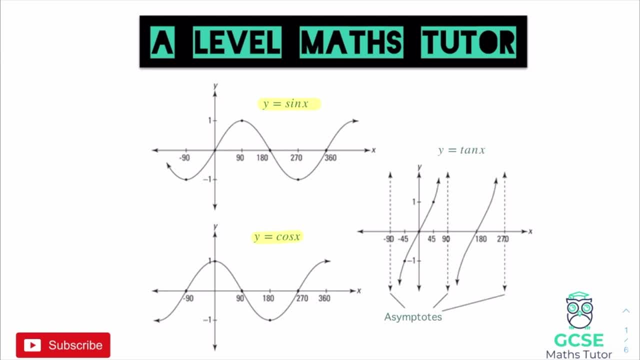 graph, which has been translated: 90 degrees to the left, So you can see. instead, it starts at 1 on the y-axis, but then it follows a very similar pattern. It goes down through 90, under 180.. Up through 270, and up and over 360. And again, this goes on infinitely to the left. 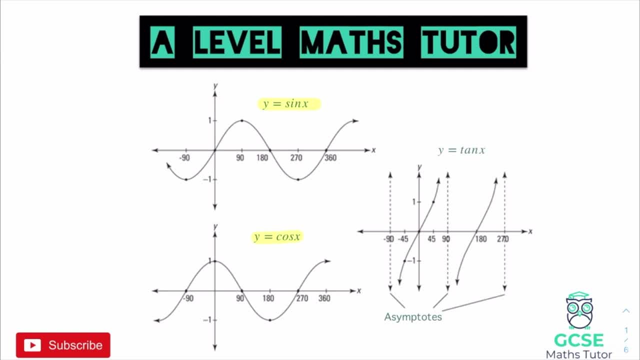 and right of the y-axis, but it follows this pattern. The tan graph is very different. It does have these waves and, as you can see, there are asymptotes at minus 90 and 90. And then each asymptote follows on every 180 degrees and 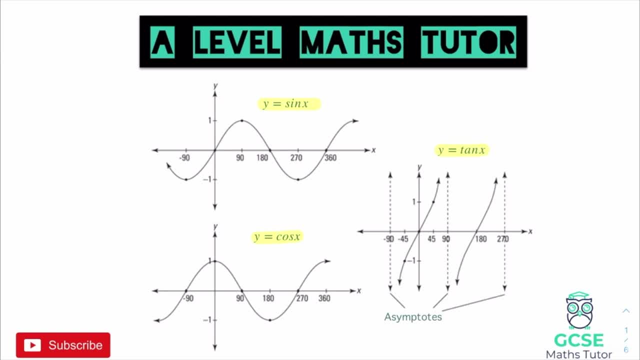 again, that is, to the right and to the left of these curves. So you do need to know these graphs, You need to be able to draw basic sketches of them, and this is going to be very helpful when we are sorting them out. 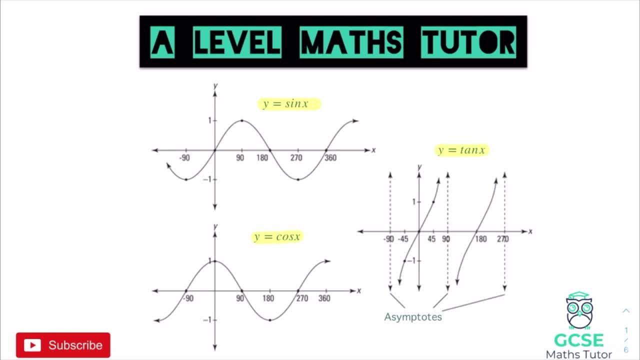 So we are going to do a very simple test of solving our trigonometric equations, as I do use a graphical method. Again. there are other ways of solving trigonometric equations, but I do use this graphical method as I do like them and I do think that it's important. 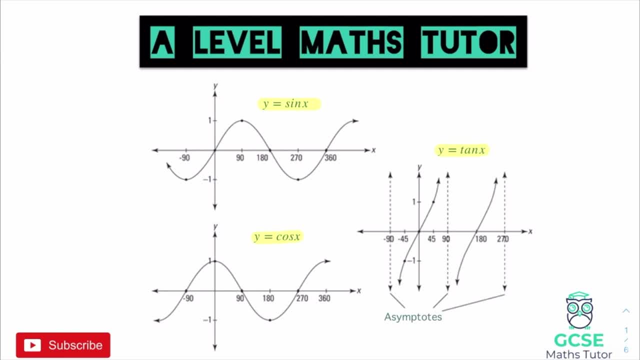 that you know these anyway, so it's always good to be able to use them for further elements. So do make sure that you can draw the equations. You can take them out on a piece of paper or you can use a pen and a pencil to draw some of the equations, But it's important that you 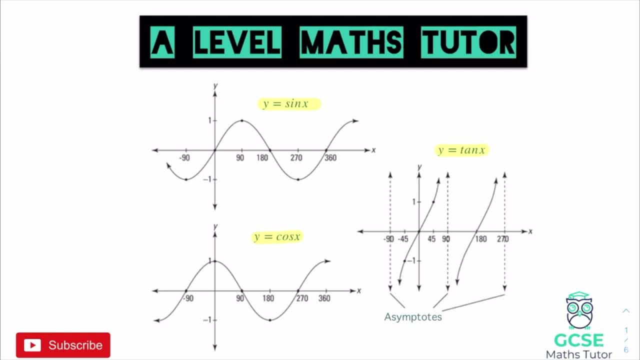 know them anyway, so it's always good to be able to use them for further elements. So do make sure that you can draw the equations, a basic sketch of all of these graphs, and you know them very well. So it says here the: 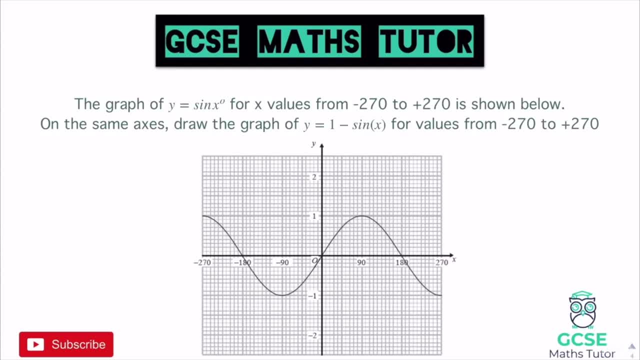 graph of y equals sin x for x values from minus 270 to plus 270 is shown below and obviously that is shown on the graph. so we've got minus 270 all the way over to 270. over here It says on the same axes, draw the graph of: and we've got y equals 1 minus sin x for values. 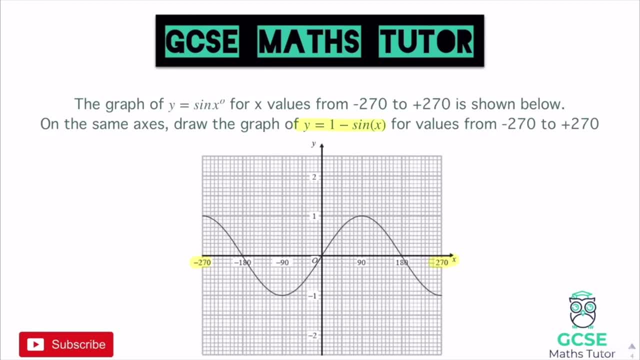 from minus 270 to plus 270.. So that's the graph we're going to have to draw there, and that doesn't look very nice. Now, this is all sort of this question here is very much linked into graph transformations. We're actually transforming this graph and we just need to. 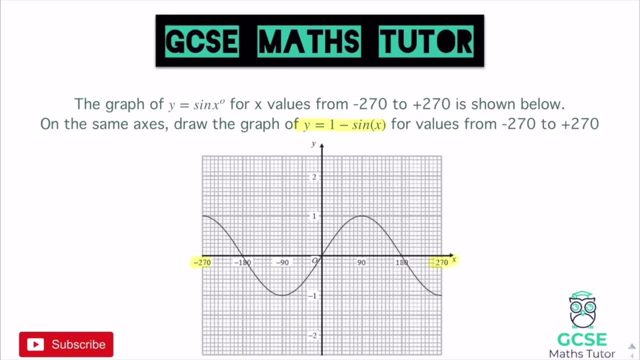 figure out how this graph is transformed, but actually we can actually do this on a calculator. Now, this particular graph transformation here has got two different transformations going on and we could rearrange that. We don't have to write 1 minus sin x, we could write negative. 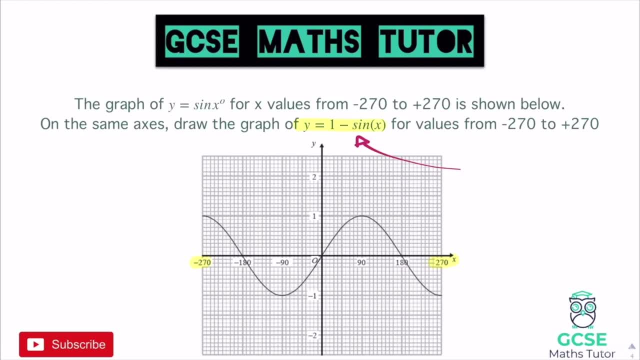 sin x plus 1 and sort of rearrange those if we wanted to. So we could do it like this: we could write: minus sin x plus 1.. Oh, missed my bracket there, let's put that back in. There we go plus 1.. And think about: 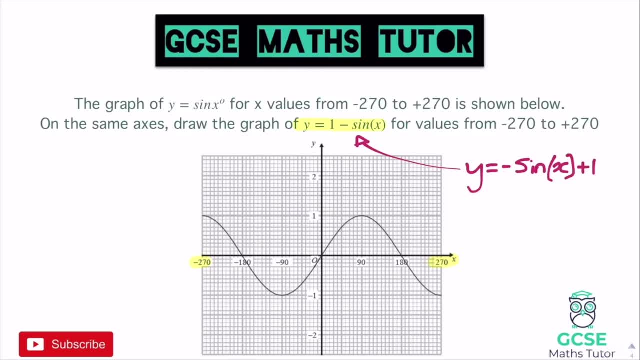 what these transformations actually represent, So that negative in front of the sin x flips the y coordinates from being positive to being negative. Obviously, check out my video- and in fact I'll link that in the description below on graph transformations as well- because it's probably worth checking out, because it does link very strongly into these trigonometric. 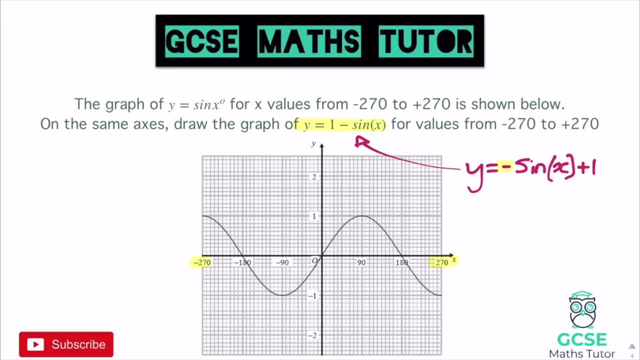 graphs. So that negative there relates to a flip or a change of the symbols. We've then got the plus 1 at the end and again that's outside the bracket. it changes the y coordinate, it changes the y intercept, it moves the whole graph up by 1.. So you could. 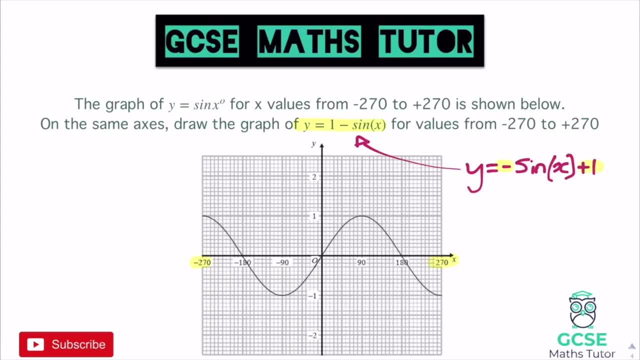 actually take a graph transformation approach to this. you could try flipping it over and then shifting it up. 1, and we could probably do that quite nice and quick. I'm going to do it in two different ways, though, but just if you are quite keen on your graph transformations. 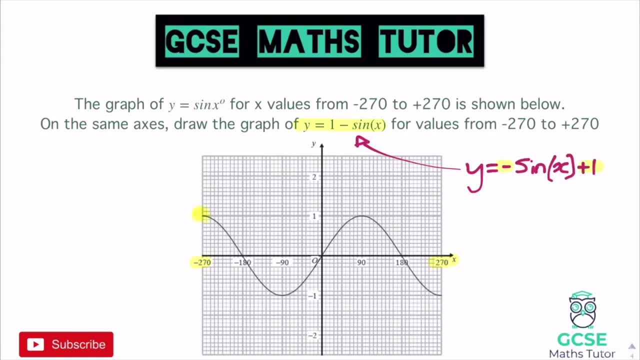 you could first flip it over and just think about that by flipping- oh, that's not my pen, let's just change that We could take all of these little coordinates here: this one, this one, this one and this one. I've not bothered with the zeros because 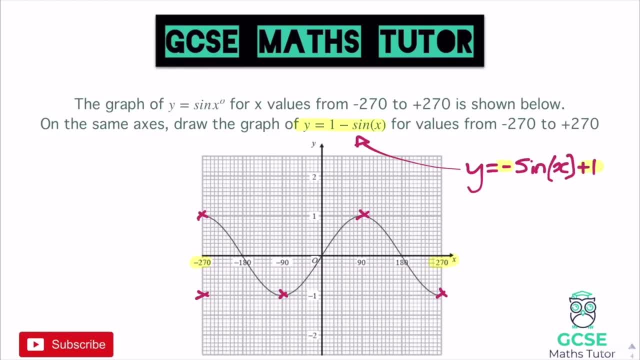 they'll stay where they are and we could just flip them down, change the coordinates there and that would move the coordinates here, and we actually end up with- and I'll try and draw it there we go, we end up with that, and then we need to shift it all up by 1.. 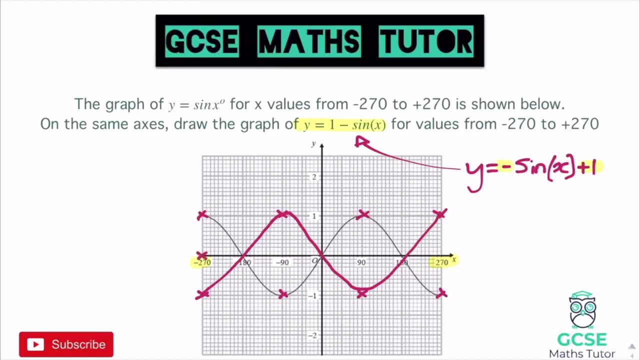 So take all those coordinates, shift them all at 1, that would shift it at 1, that would shift it at 1,. let's have a look: these zero coordinates need shifting at 1 as well. try and shift them all at 1,. it's not the nicest now when you start drawing all over this there. 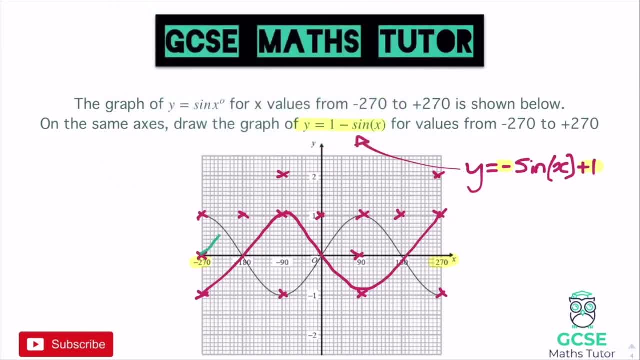 we go, shift that all at 1 and it makes this sort of curve here. there we go. so drawing it using a graph transformation approach, let's just get rid of that red one. there we go. that is where our curve ends up following this graph transformation. 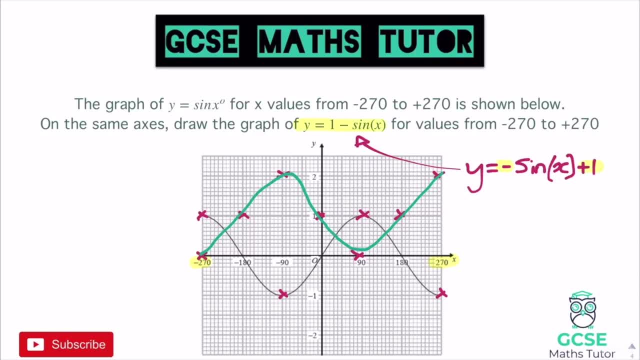 Not the nicest, though that's quite nasty actually. it's a very sort of horribly difficult graph transformation question, having to sort of flip it over the x-axis there and then actually shift it at 1 as well. but I'm going to take a little bit of a different approach. 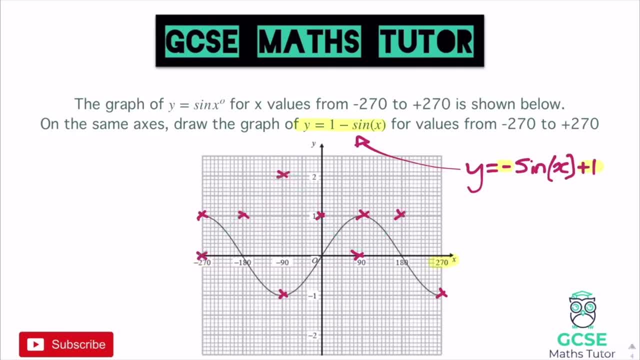 But just so you know, you could actually take that approach there using graph transformations. so obviously check that video out. if you're not sure on that, you can always have a think about what I've actually done there once you've had a look at that. 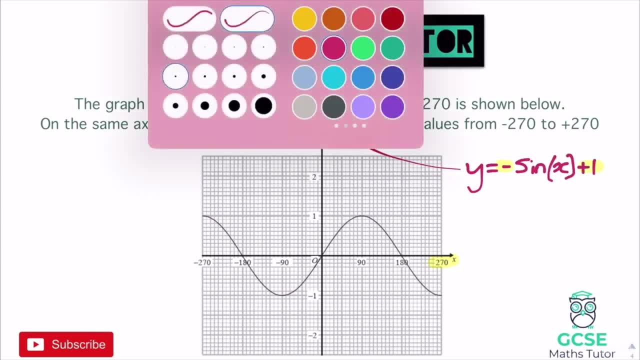 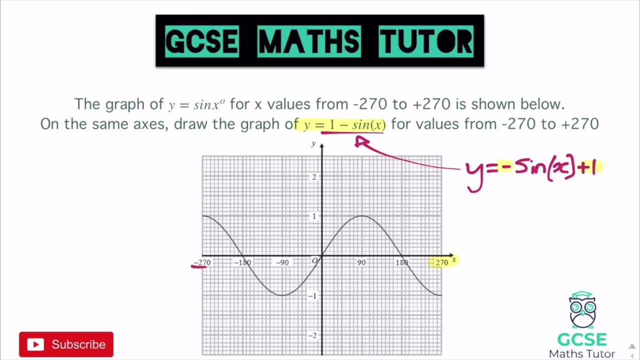 Now, instead of doing that, I'm just going to take this nice calculator approach, because this was actually a calculator question as well. So, rather than doing that, I'm just going to plug my numbers into this formula here. so I'm going to start with negative 270, so I'm going to do 1, take away and I'm going 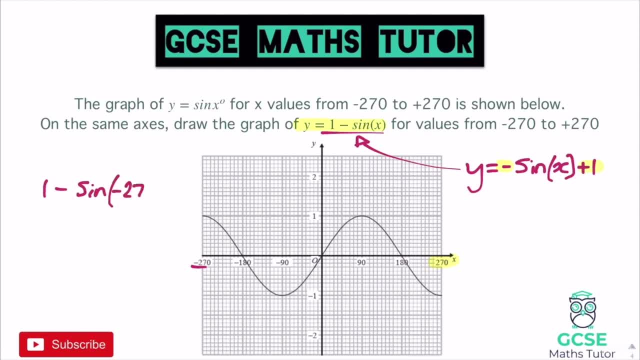 to do sine minus 270,. there we go, And that's going to give me my first value, so 1,. take away sine and I'll put minus 270 in the bracket and I get the value of 0, there we go. so that's my 0.. 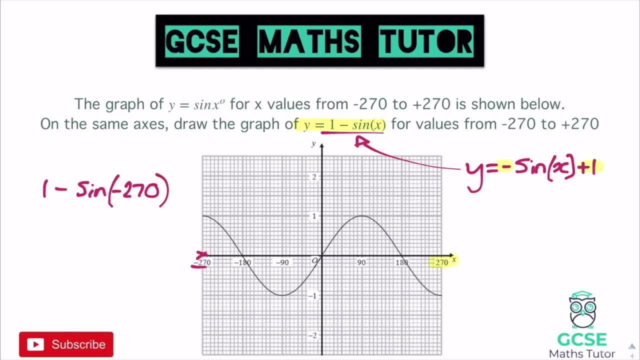 Then I'm just going to change that for the negative 180, so I'm just going to put minus 180, I'm just going back into my calculator and changing that value and that gives me that value there Back in negative 90, there we go and that gives me 2, so negative 90 is up here at 2.. 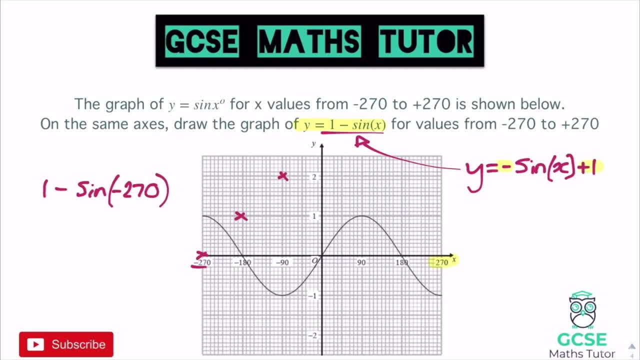 I'll put 0 in, And that gives me 1, there we go. put 90 in, and that gives me sorry. I'll put that in: 1 minus 90, yeah, that gives me 0, there we go. 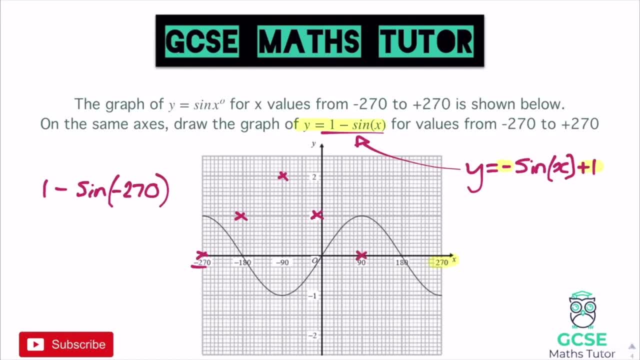 Then put 180 in last one, nearly done, and that gives me 1,. where's that gone? 1 is there. and then 270,. there we go, and that gives me 2, and that is there. Again, just drawing that up with a nice smooth curve as best you can. there we go, and there. 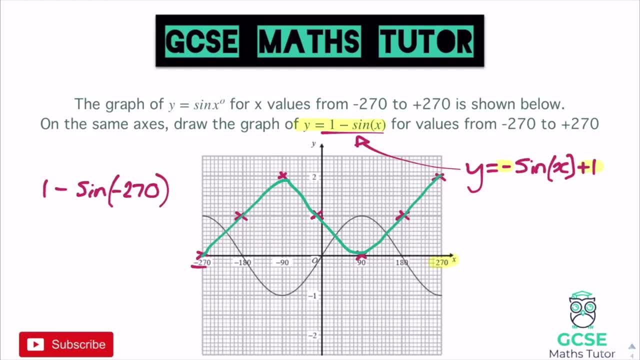 is our transformed graph. Again, two different methods that you could take to approach that. Obviously, if you're really good with your graph transformations, you could have flipped it over first, changed the y coordinates, made them positive and negative, and the negative 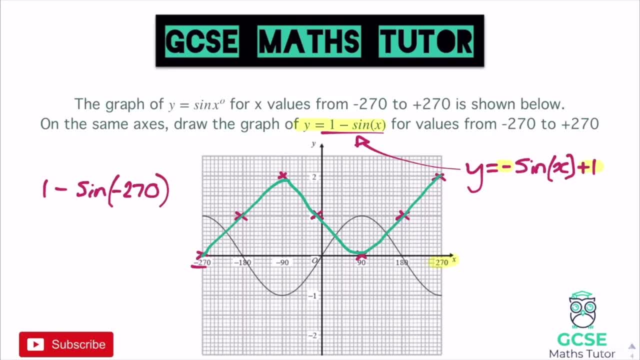 one's positive and then obviously shifting it up, one, doing that transformation with the one at the end, changing the y intercept. or you could just take this approach: just plug in the numbers into the calculator, plot them all nice and neat and connect them all. 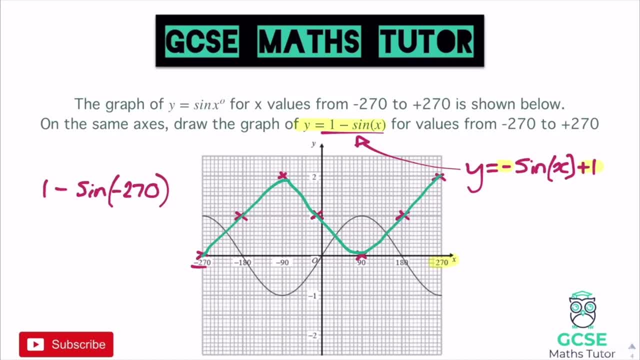 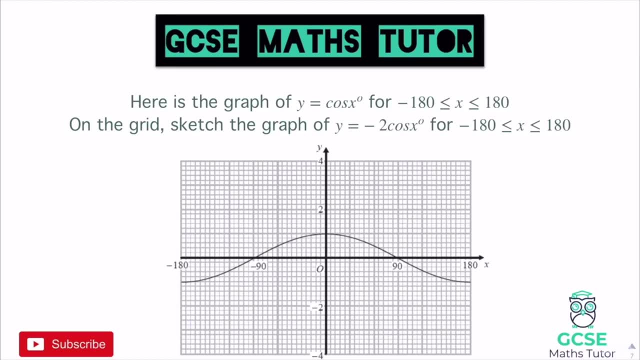 up together. It's up to you which one you prefer- Just a couple of different ways that you can actually approach that question. This says: here is the graph of y equals cos x between the values minus 180 and 180, and: 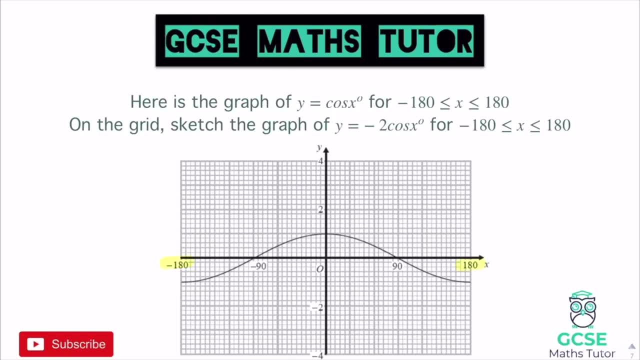 again, we can see that on the graph it does stretch from minus 180 to 180.. It says on the grid: sketch: the graph of y equals negative 2 cos x. but again, between these values, Taking a little approach to this, then I'm just going to take the calculator approach. 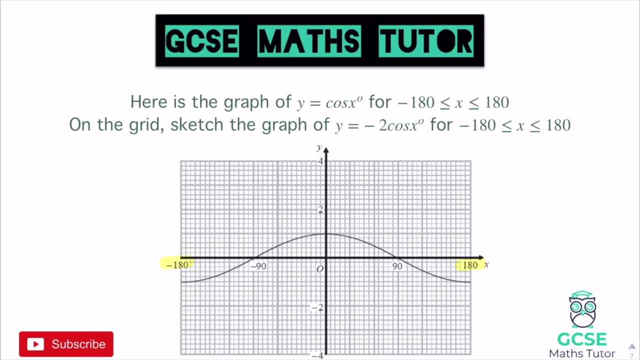 Again, you could take a graph transformation approach to this. but let's have a look at the end and see what happens. Let's see what that graph transformation is. We'll take that calculator method to start with and just start plugging the values into. 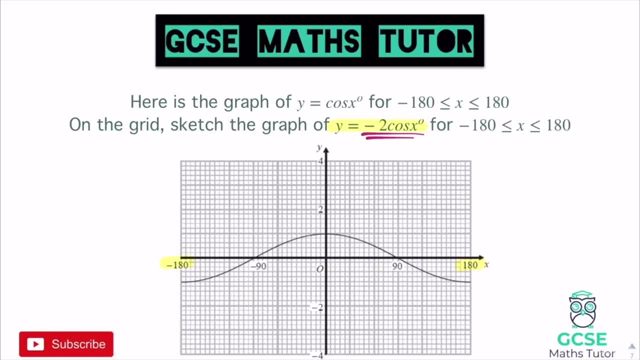 this formula We've got: y equals negative 2 cos x. so on my calculator I'm just going to type in negative 2 cos and I'm going to start with that first value on the x there, which is negative 180.. 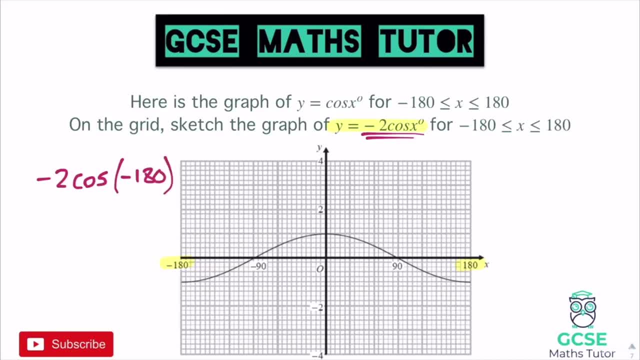 So minus 2 cos, and then negative 180 in the bracket, and it gives me the value of 2.. There we go, that equals 2, and I'm just going to do that same approach for all of them, so that 2 goes up to 180. 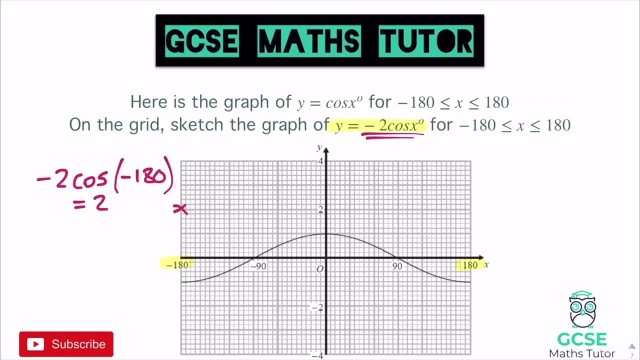 It goes up to there and there we go. So back into the calculator. I'm not going to sort of do all the little sub-values in between, I'm just going to go straight for negative 90 and see where that is. So negative 90 ends up at 0, and there we go. so that stays where it is. 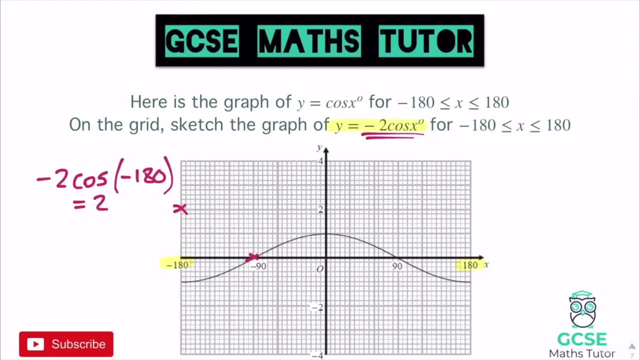 I'm going to go for 0 now. so back in negative 2 cos 0, and that gives me a value of negative 2.. Let's go back for 90,. negative 2 cos 90 gives me a value of 0, and negative 2 cos 180 gives. 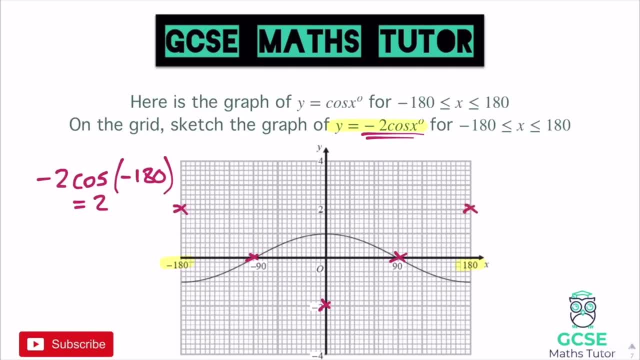 me a value of 2.. There we go. So that value of 2 is there and again we just need to join that up with a nice smooth curve. There we go and that's our point drawn there. So again, that's one method that you could approach. 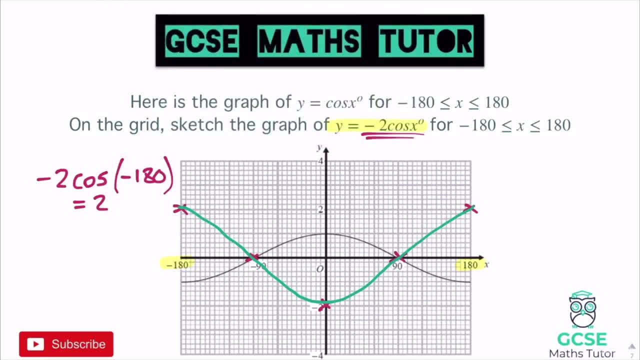 If I swap to a different colour here, we'll have a think about the graph transformation as well. So negative: there flips the coordinates over, so I could have actually started by flipping those coordinates over, so let's go about doing that. We've got this one here which is going to flip to the other side there. 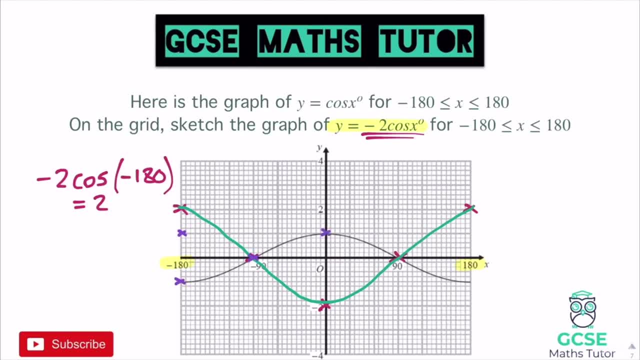 Zero stays. that one there stays where it is. This one here on 1 flips down to minus 1. Which we can just about see. it's about there somewhere. We've got the one on the axis there which stays where it is, and we've got this one. 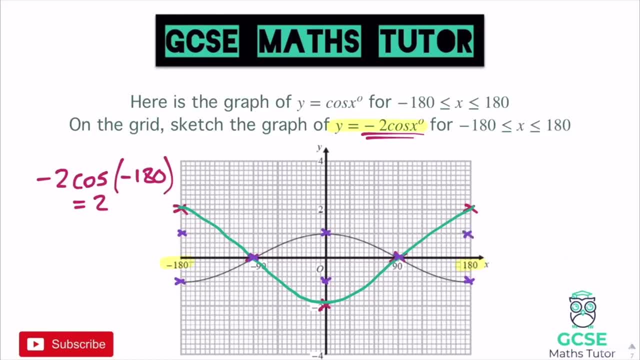 down here which flips up above. So the minus part, just like before, changes the symbols in front of the y-coordinates, So we can draw that in. I'm going to get rid of this in a sec and just about draw that.